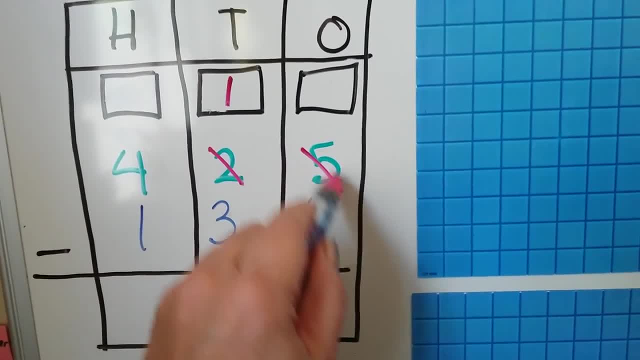 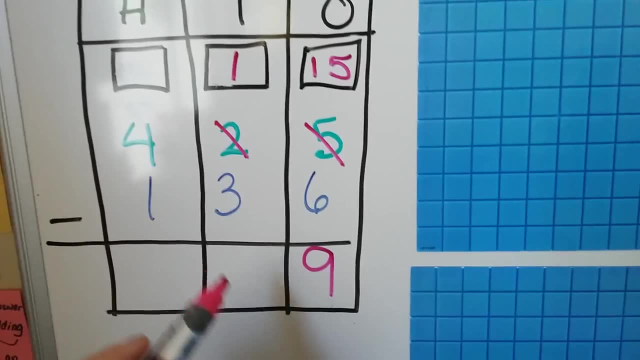 I'm going to give that 10 to the ones place. so this is not a 5 anymore, it's a 15.. 15 take away 6 is 9.. Now we have 1, and we need to take 3 away, but we can't do that. 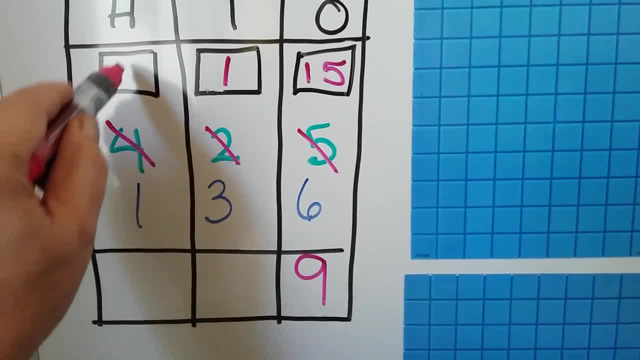 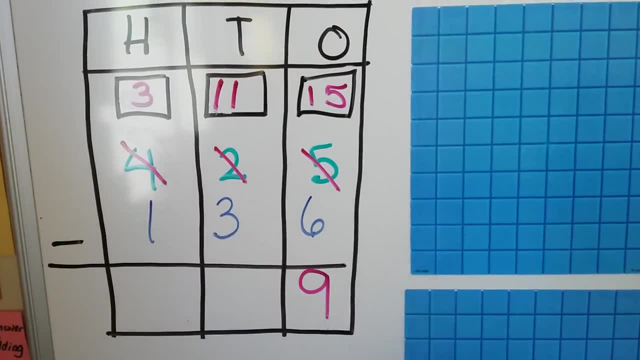 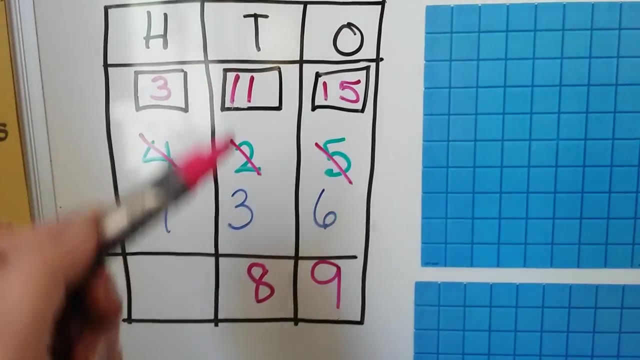 So we regroup this to be a 3, and we give it to the tens place. Now we have 11 tens and we need to take 3 away. That's an 8.. 8,, 9,, 10, 11.. See, 8 plus 3 is 11.. We can do the opposite, We can do addition to check our subtraction. 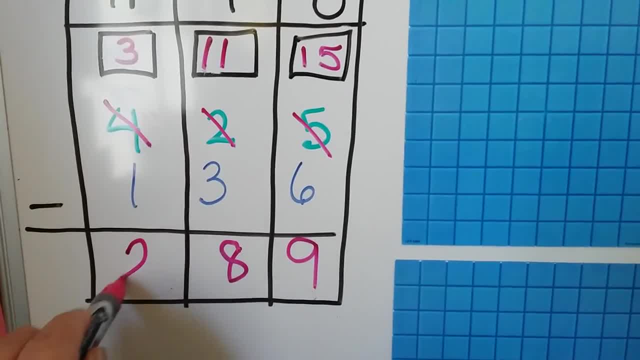 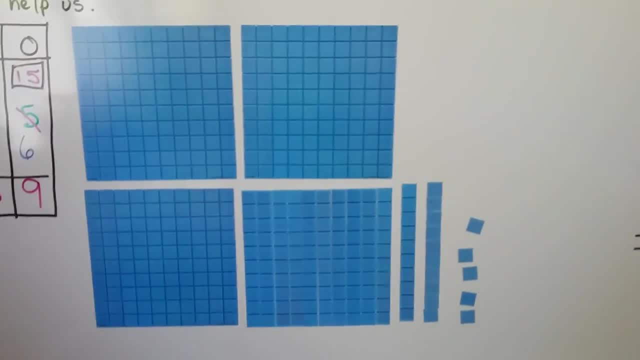 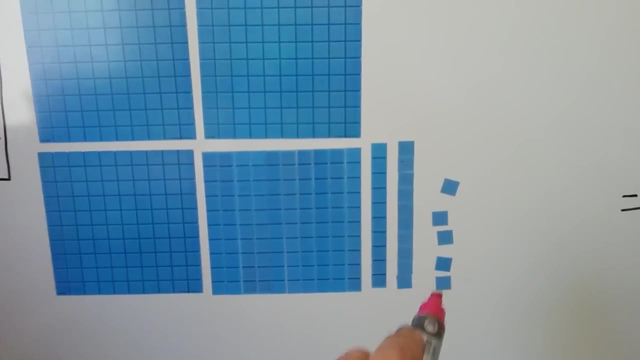 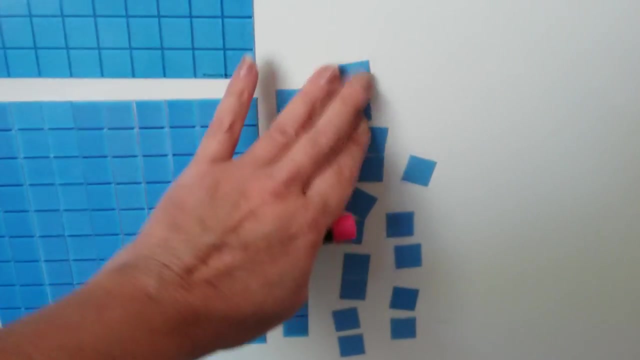 3 minus 1 is a 2, so we should have 289.. So let's see how this works. We had 425 here and we need to take away 6 ones. right, But we can't take away 6 ones because there's only 5 ones there. So what we can do is we can break this 10 up into ones and regroup it to be ones. See. 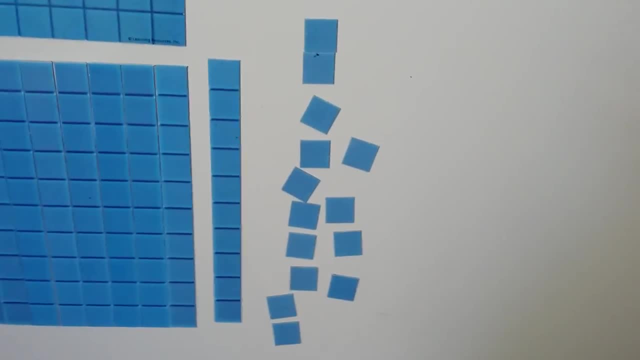 Now we can take 6 of them away. Now we can take 6 of them away: 1,, 2,, 3,, 4,, 5, 6.. We take 6 of them away, and how many ones are left? 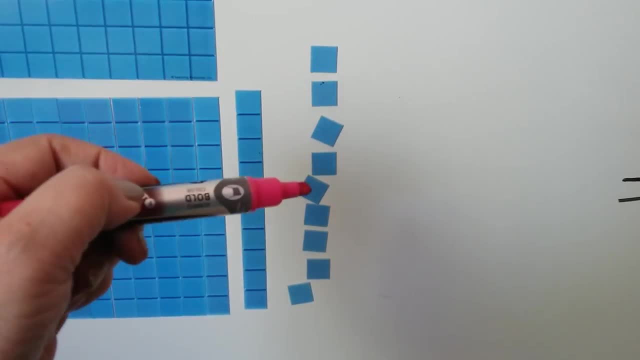 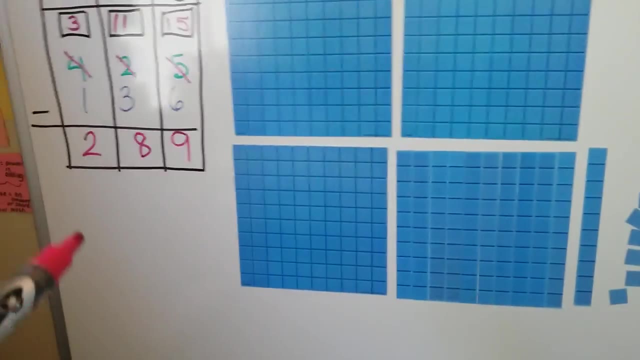 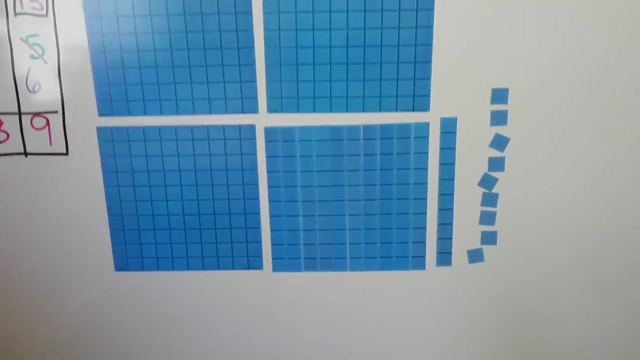 1,, 2,, 3,, 4,, 5,, 6,, 7,, 8, 9.. Just like we got here, We have 9 ones. Now. it says that we have to take away 3 tens, but I only see one ten here. 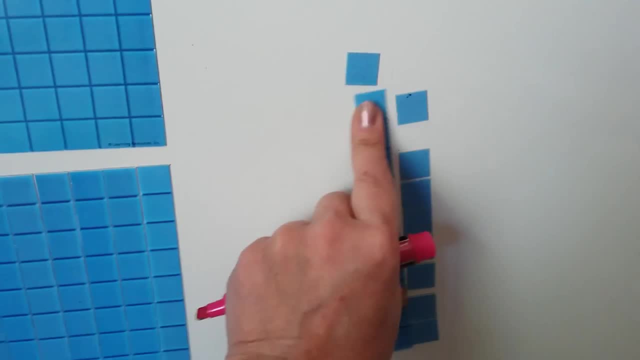 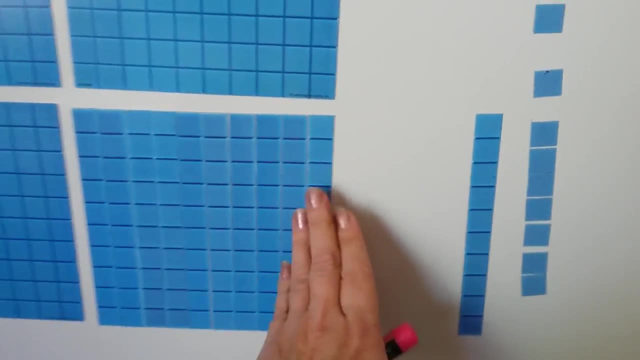 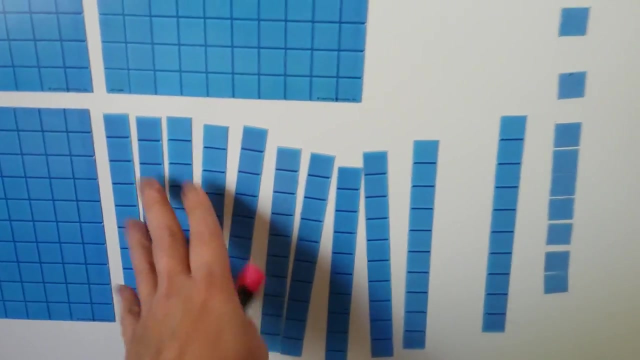 So what we can do is can move our ones over and out of the way a little bit. We only have one ten here. We can split this hundred up as ten tens See, And regroup it to the tens place. Now we have one, two, three, four, five. 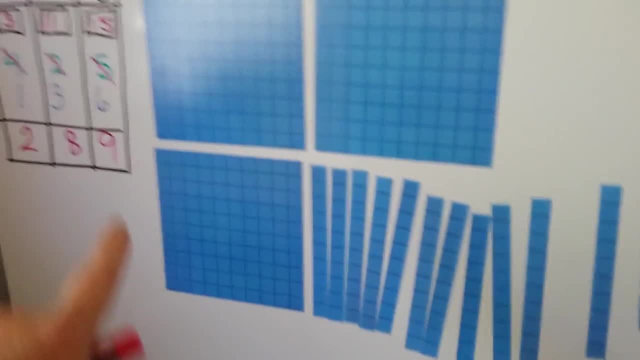 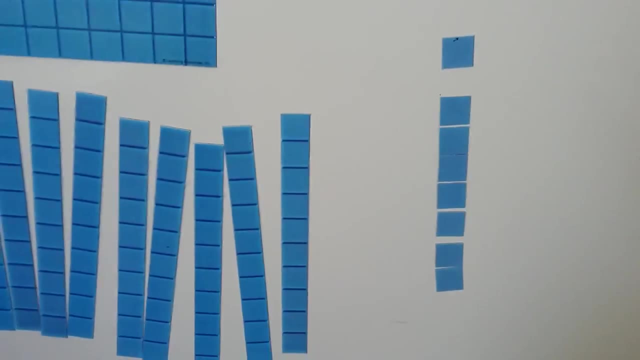 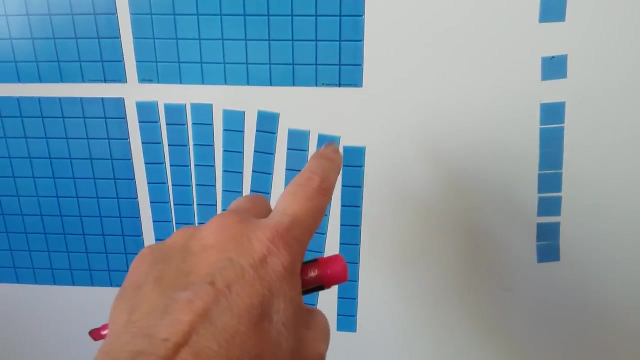 six, seven, eight, nine, ten, eleven tens. Just like we got up here, We have eleven tens. Now we can take three away. We can take away one, two, three, and we're left with one, two, three, four, five, six, seven. 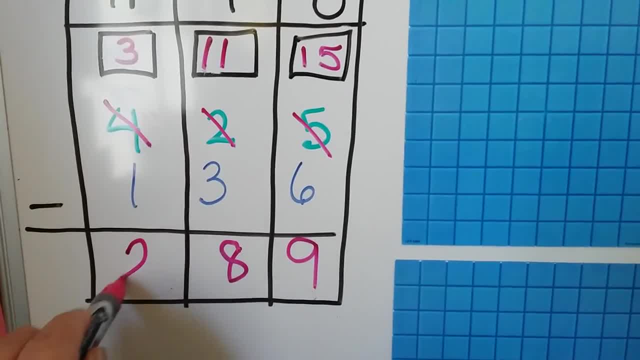 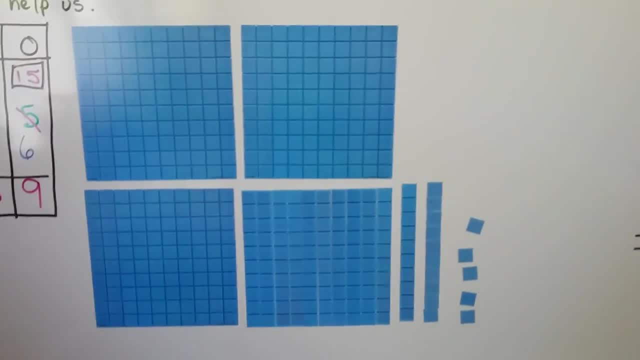 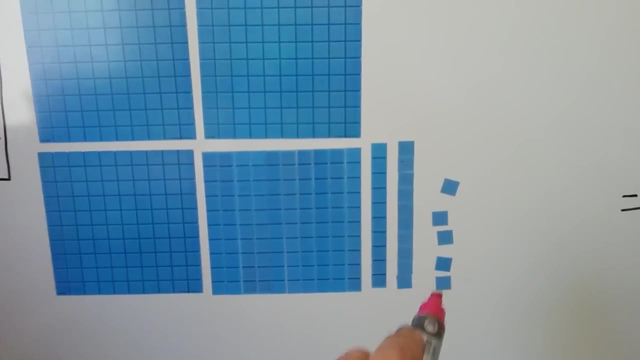 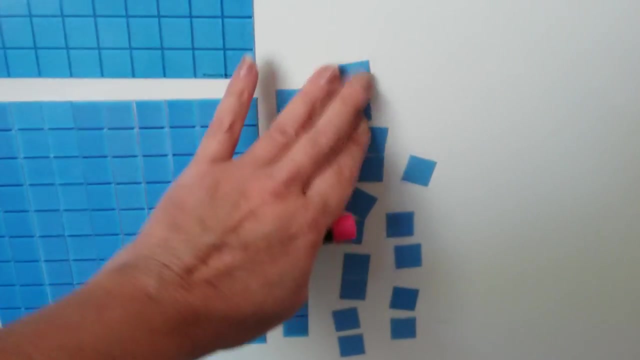 3 minus 1 is a 2, so we should have 289.. So let's see how this works. We had 425 here and we need to take away 6 ones. right, But we can't take away 6 ones because there's only 5 ones there. So what we can do is we can break this 10 up into ones and regroup it to be ones. See. 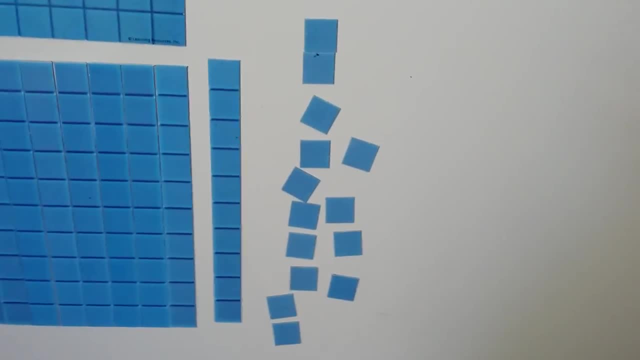 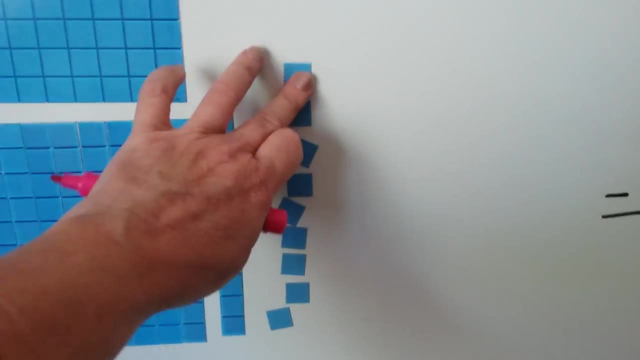 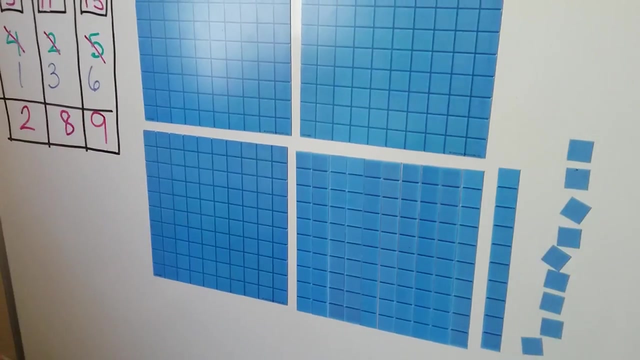 Now we can take 6 of them away: 1,, 2,, 3,, 4,, 5, 6.. We take 6 of them away, and how many 1s are left? 1, 2,, 3,, 4,, 5,, 6,, 7,, 8, 9.. Just like we got here. 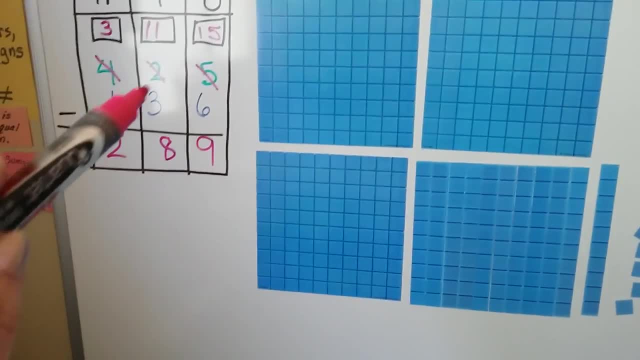 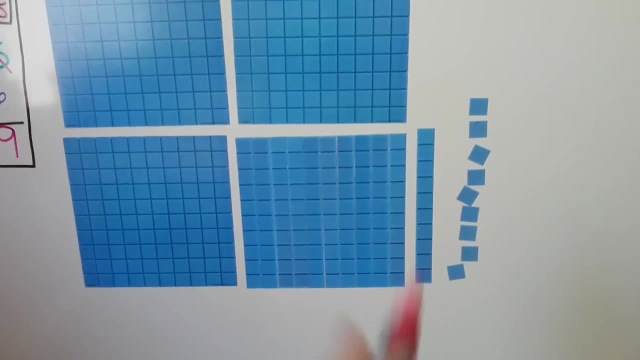 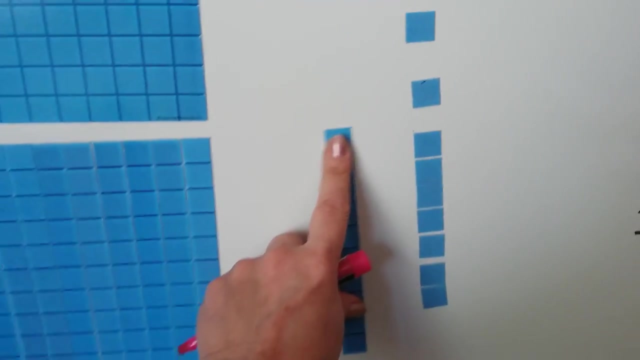 9 ones. Now it says that we had we have to take away 3 tens, But I only see 1 ten here. So what we can do is we can add a new, can move our ones over and out of the way a little bit. We only have one ten here. We can split this. 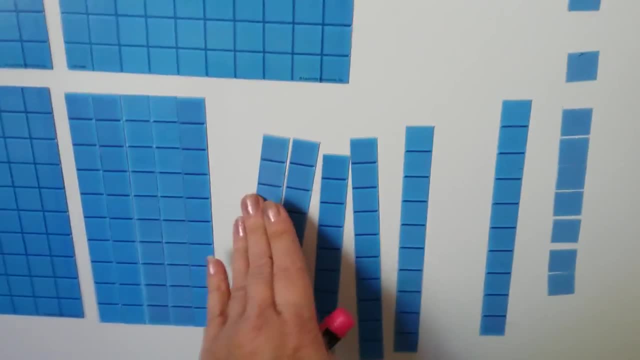 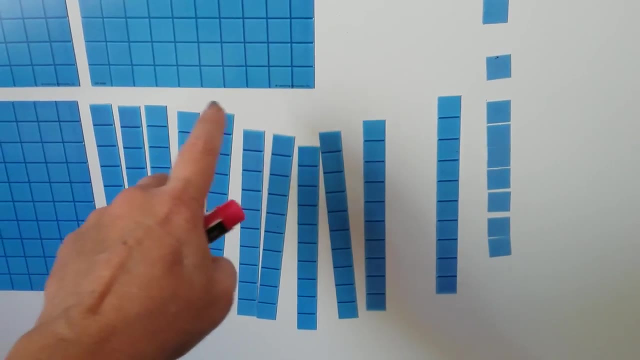 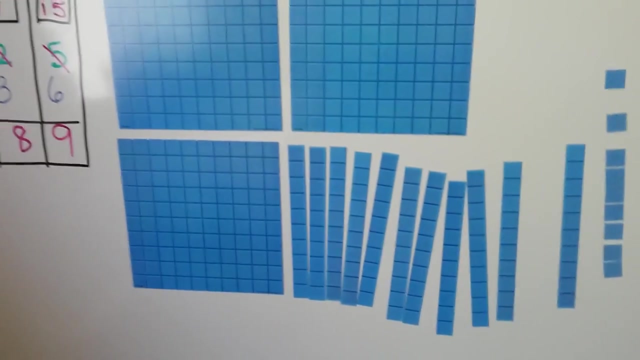 hundred up as ten tens See And regroup it to the tens place. Now we have one, two, three, four, five, six, seven, eight, nine, ten, eleven tens. Just like we got up here, We have eleven tens. Now we can take. 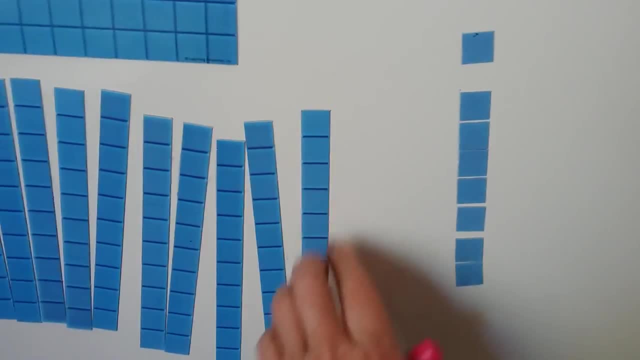 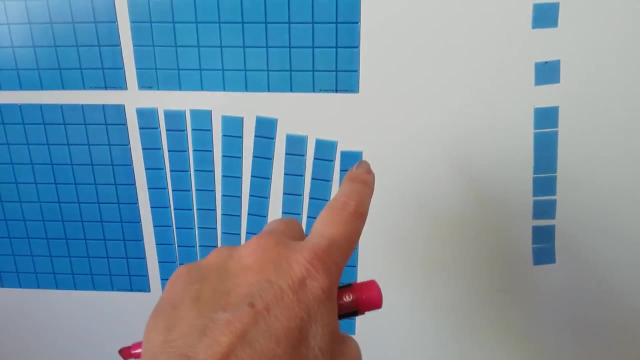 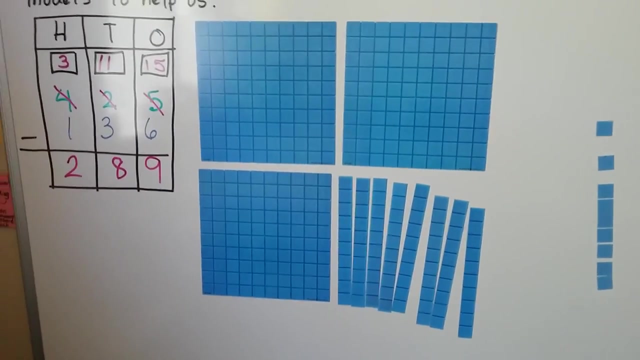 three away. We can take away one, two, three, and we're left with one, two, three, four, five, six, seven, eight tens, Eight tens and nine ones, Just like we got when we did the math. Now it says we need to. 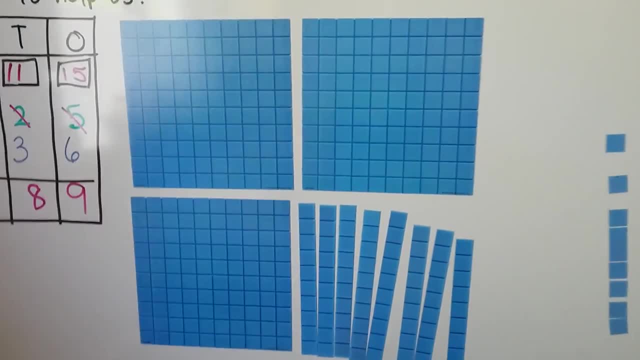 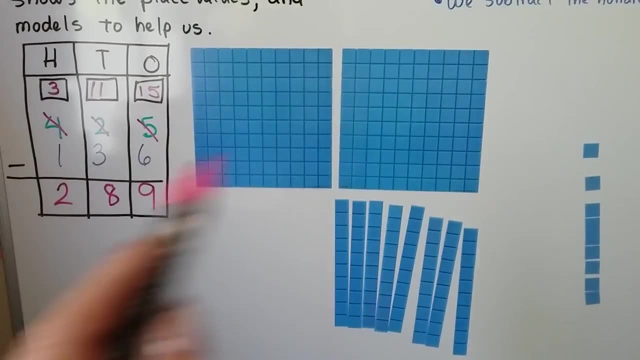 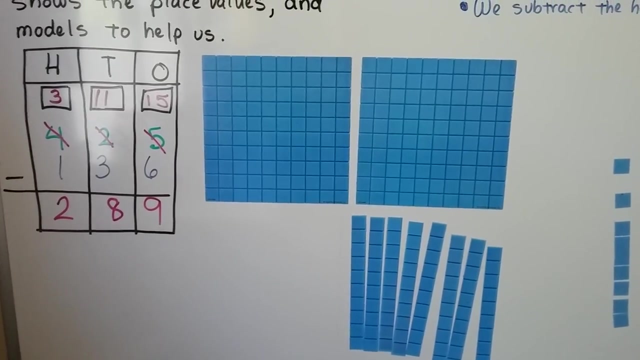 take away a one hundred. Well, if I take away a one hundred, that's one of these big squares. what are we going to be left with? Two hundreds, See, Eight tens and nine ones, Just like we got there, See. So if you need to use models, that's. 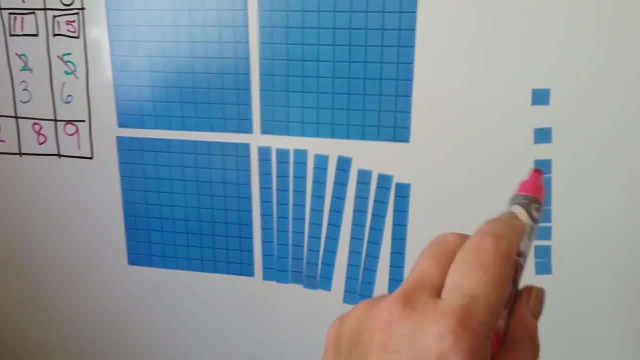 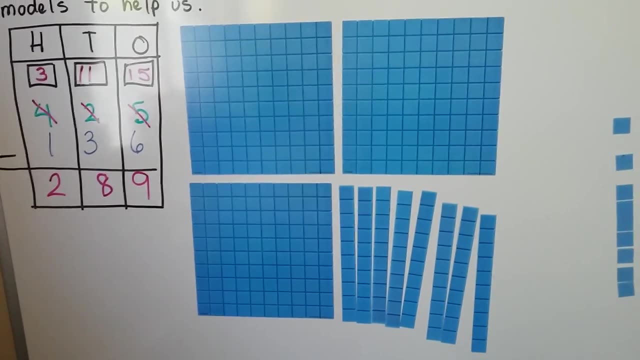 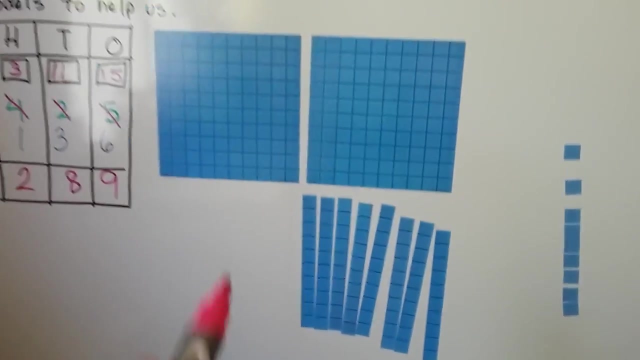 eight, tens, Eight tens and nine ones, Just like we got when we did the math. Now it says we need to take away a one hundred. Well, if I take away a one hundred, that's one of these big squares. what are we going to be left with Two hundreds? 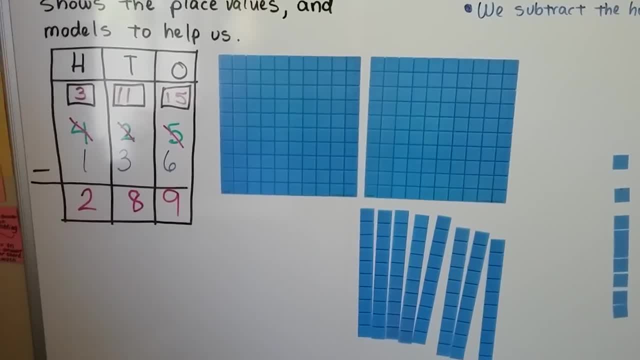 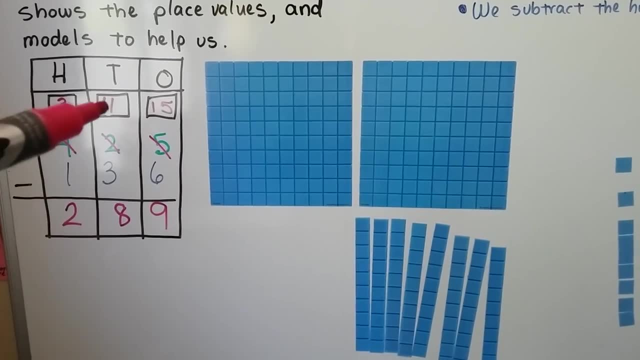 See Eight, tens and nine ones, Just like we got there, See. So if you need to use models, that's okay, And you can use a work mat like this that has little boxes for your regrouping, Alright, So let's. 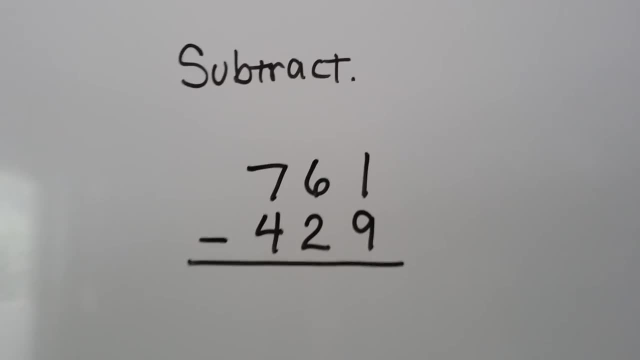 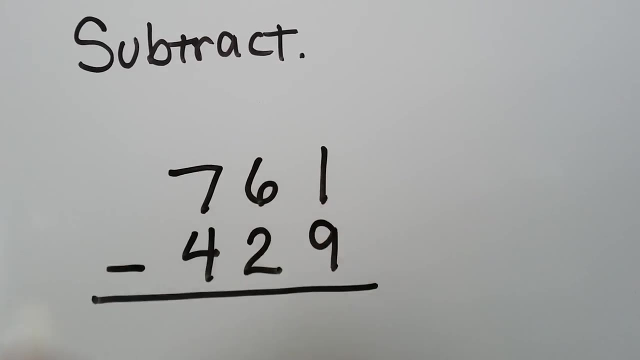 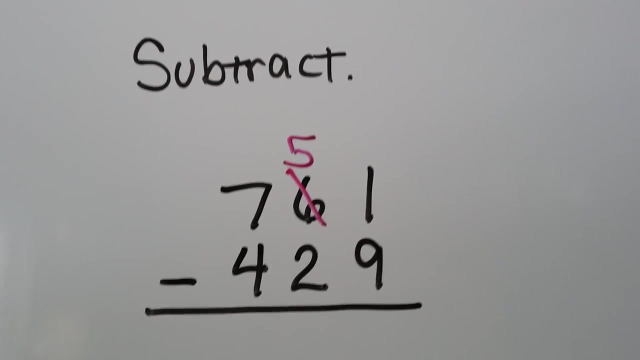 see if we can subtract these. We have seven hundred sixty-one and we need to take away four hundred twenty-nine. We have one and we need to take away nine. Well, we can't because the nine's so big. So let's see if we can subtract these. We'll turn this into a five And we're going to give the ten to the one's place. 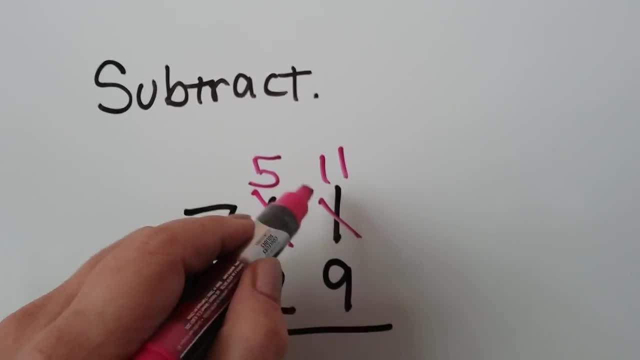 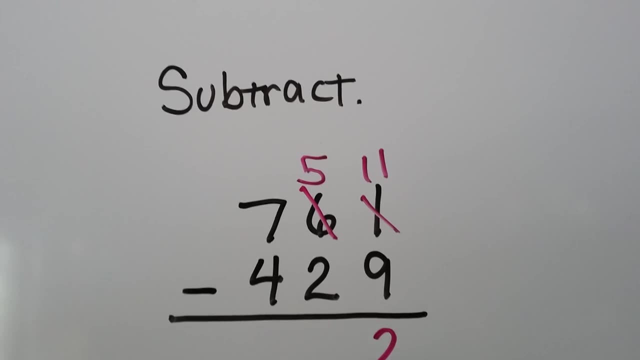 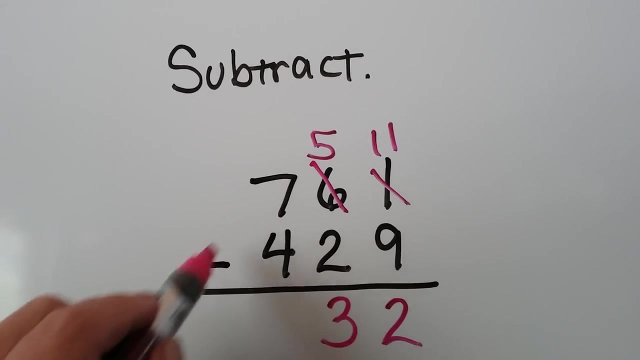 So now, instead of one, we have eleven, Because ten plus one is eleven, isn't it? Eleven minus nine is a two, right? Five minus two is a three, And seven minus four is a three. See, So we had to regroup two times, didn't we? But that's. 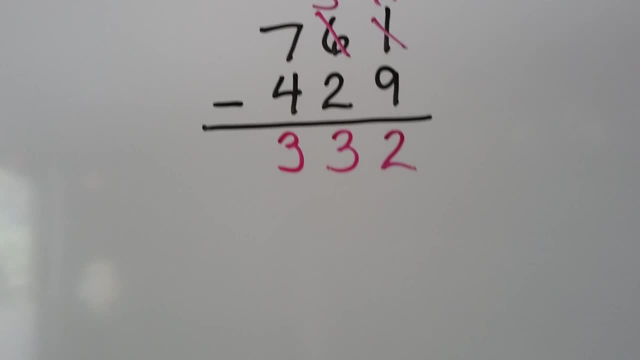 okay, We can do that. We can regroup many, many times if we have to in a math problem. Let's try this one. We have five hundred seventy-four and we need to subtract two hundred twenty-eight. So in the one's place we have a four and we need to take away an eight and we can't because the eight's. so 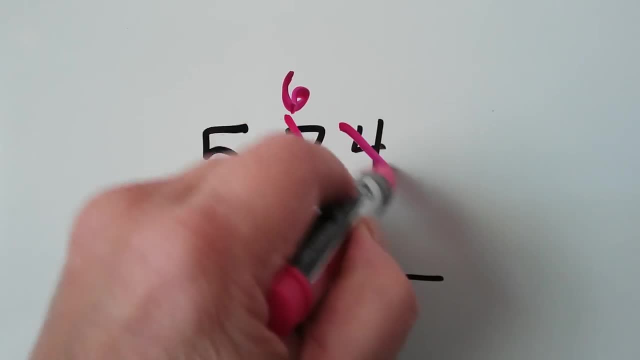 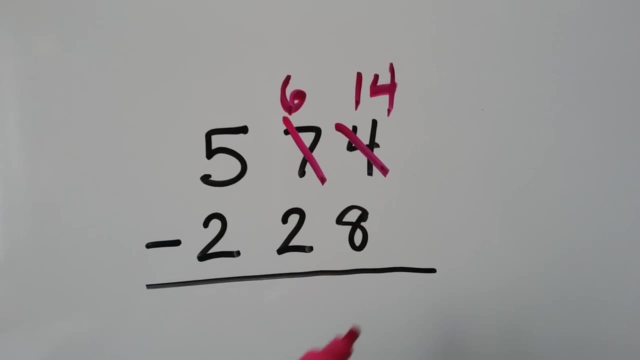 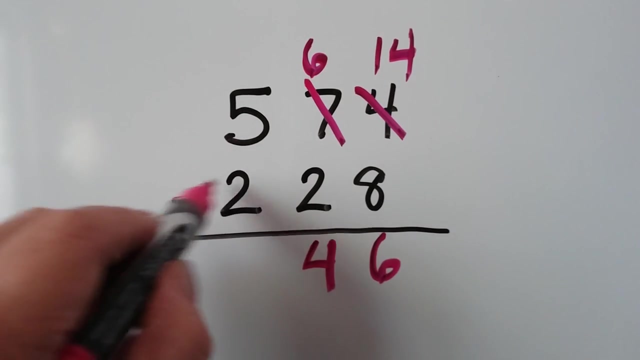 big. So we're going to turn this into a six and regroup our four ones into fourteen ones, Because if you said six, you're right. Six take away two is four, And five take away two is three. We have three hundred forty-six. 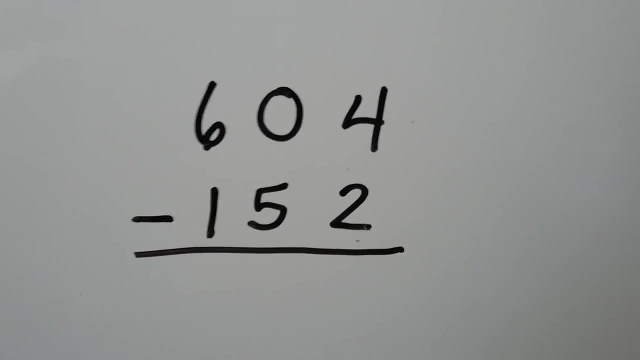 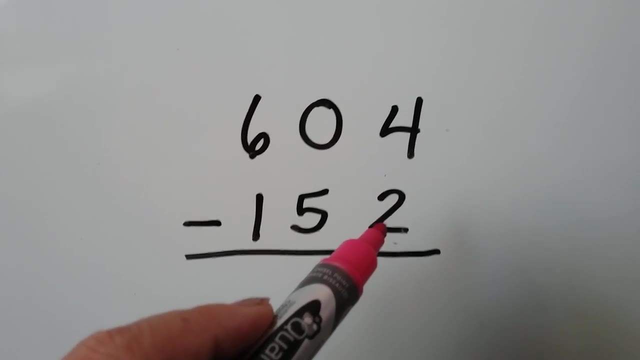 Alright, let's try this one. We have six hundred four and we need to subtract one hundred fifty-two. We have four. take away two, We can do that. We don't need to regroup. That's a two, isn't it? 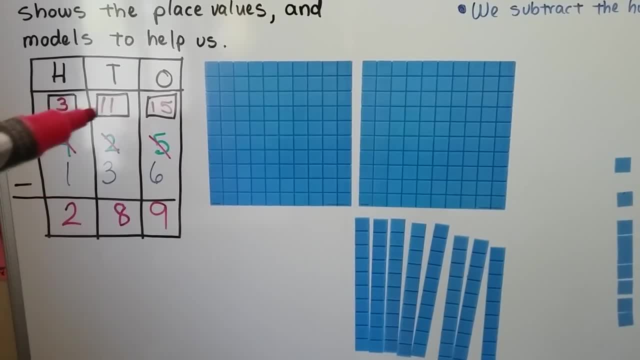 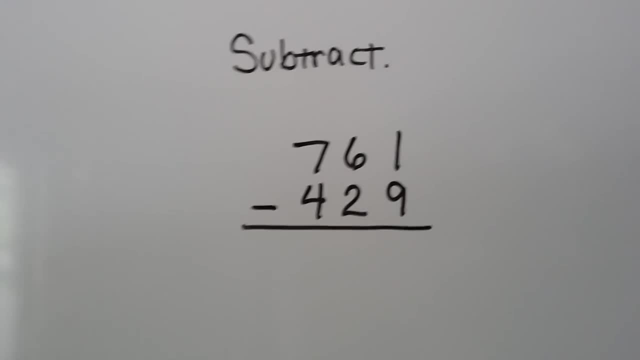 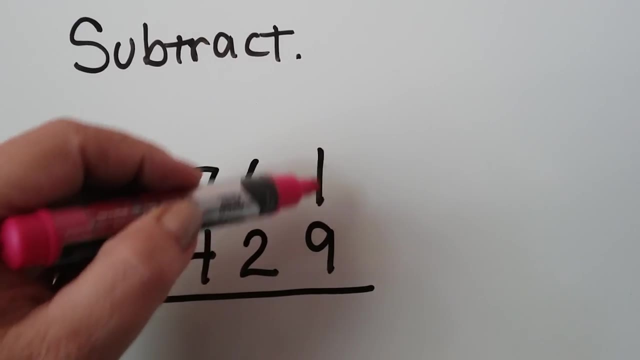 okay, And you can use a work mat like this that has little boxes for your regrouping. Alright, So let's see if we can subtract these. We have seven hundred sixty-one and we need to take away four hundred twenty-nine. We have one and we need to take away nine. Well, we can't because the nine's so big, So let's. 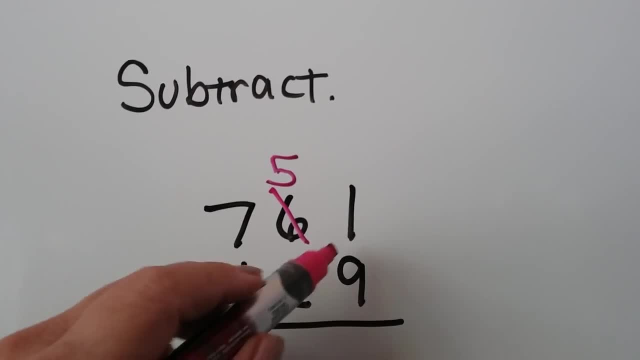 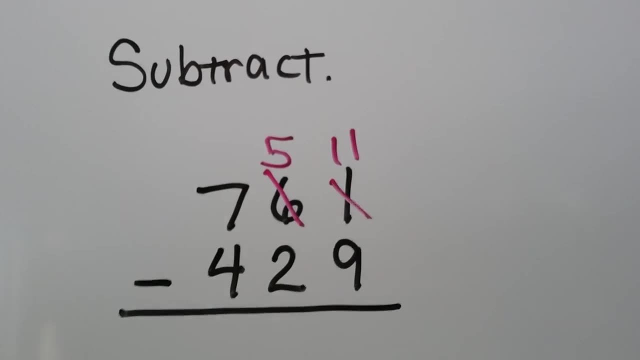 see if we can subtract these. We'll turn this into a five And we're going to give the ten to the one's place. So now, instead of one, we have eleven, Because ten plus one is eleven, isn't it? Eleven minus nine is a two, right. 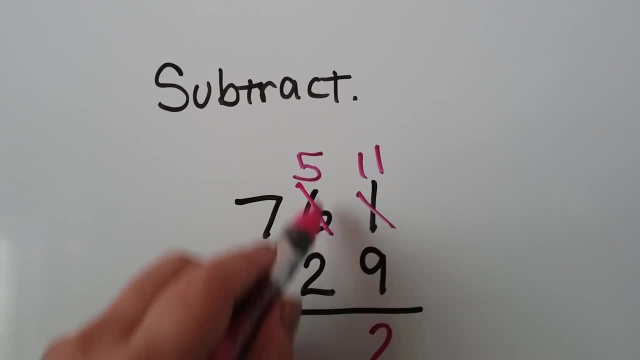 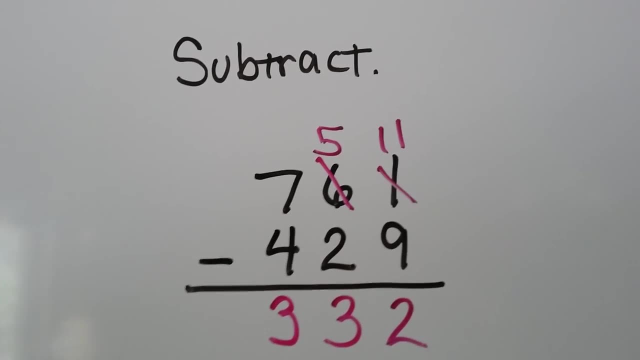 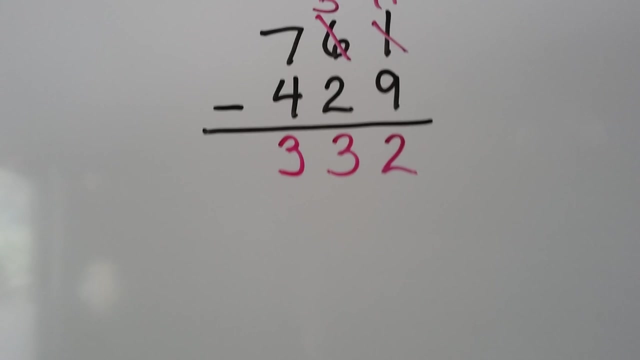 Five minus two is a three, And seven minus four is a three. See, So we had to regroup two times, didn't we? But that's okay, We can do that. We can regroup many, many times if we have to in a math problem. Let's try. 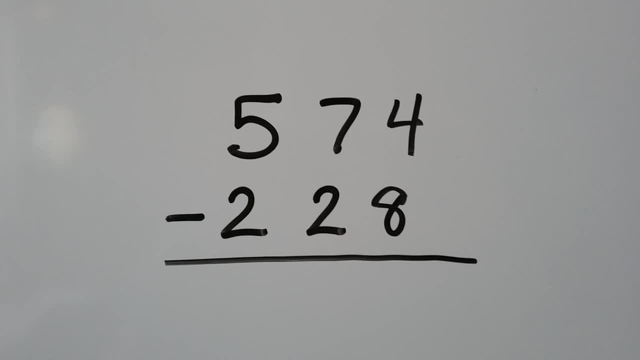 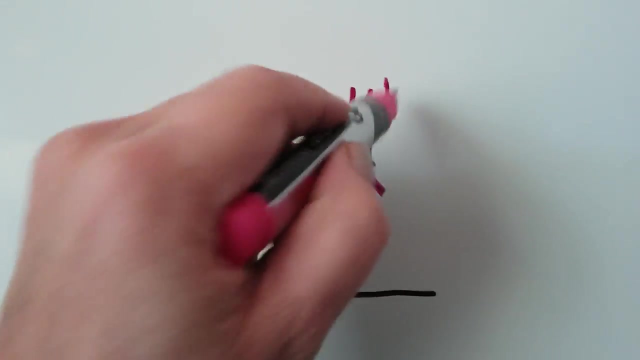 this one, We have five hundred seventy-four and we need to subtract two hundred twenty-eight. So in the one's place we have a four and we need to take away an eight and we can't because the eight's so big. So we're going to turn this into a six and regroup our four ones into fourteen ones, Because 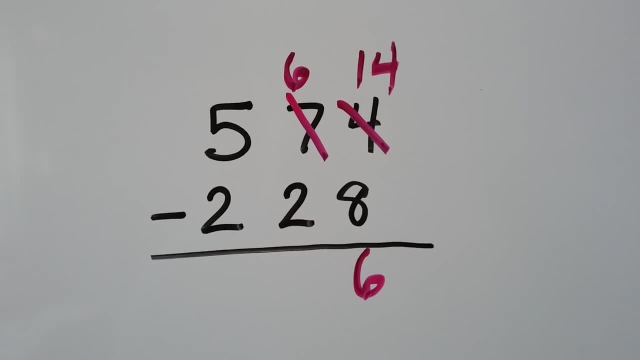 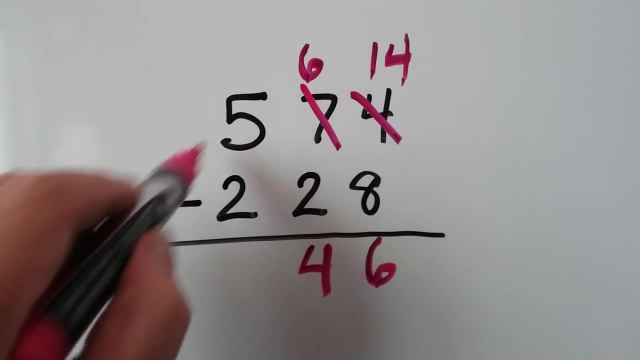 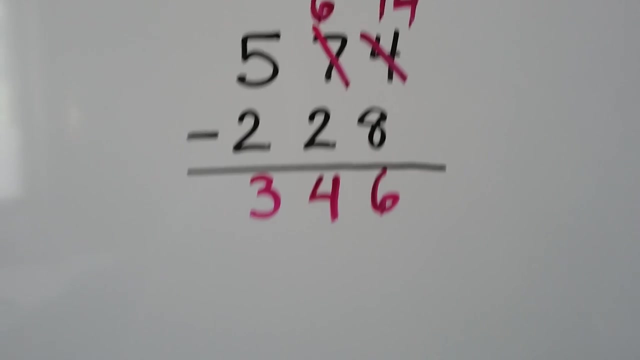 if you said six, you're right. Six take away two is four, And five take away two is three. We have three hundred forty-six. Alright, let's try this one. We have six hundred four and we need to subtract one hundred fifty-two. We have four, take away two. 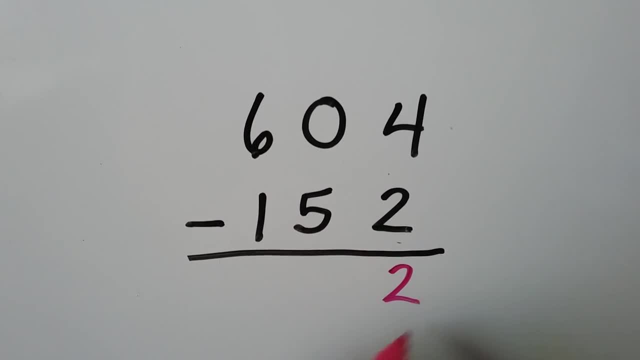 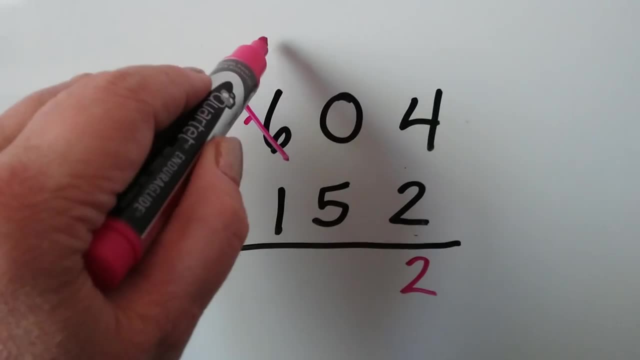 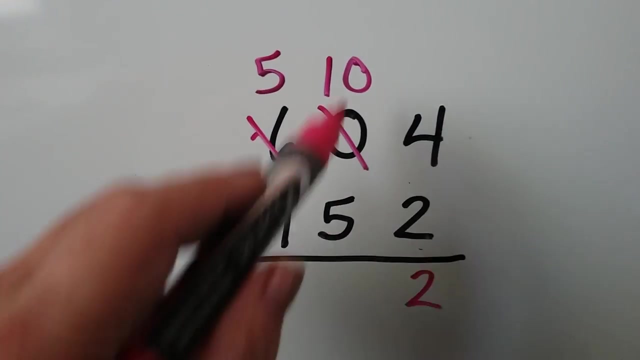 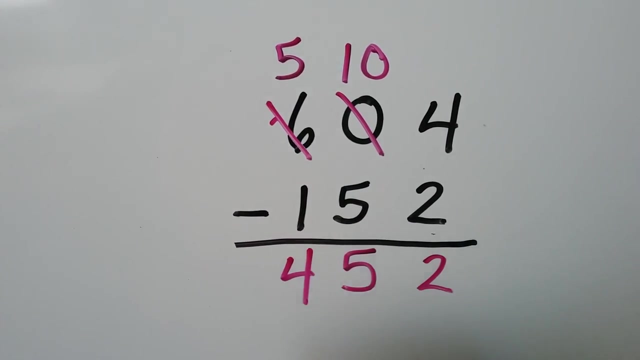 We can do that. We don't need to regroup. That's a two, isn't it? We have zero. take away five. Oh, we need to regroup because that zero is too small. This becomes a five. We give that to the tens place Ten tens make a hundred. So we have ten tens now. Ten take away five is five, And five take away one is four. We have four hundred fifty-two. 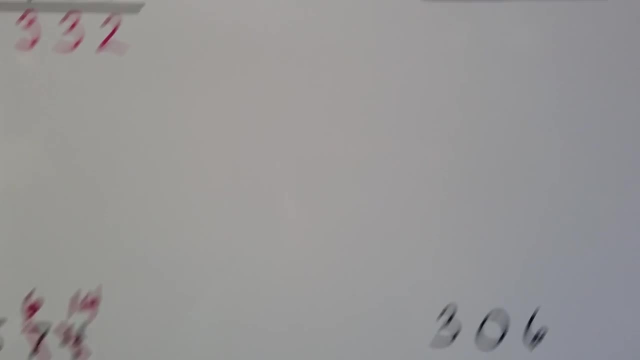 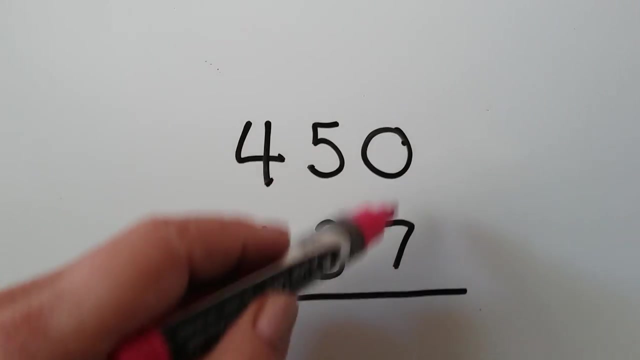 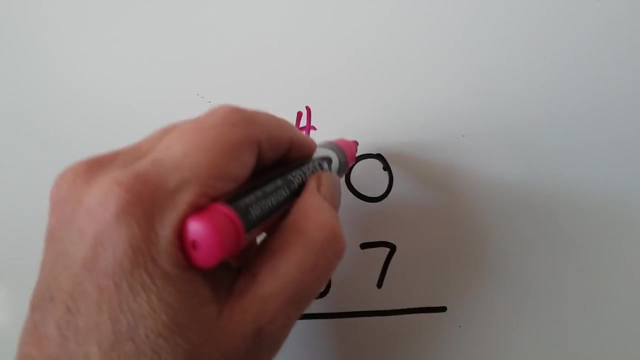 Alright, let's try it again. We're going to get lots of practice. We have four hundred fifty And we need to subtract one hundred thirty-seven. We can't have zero and take seven away, So we're going to regroup. This is going to become a four And we're going to give that ten to the ones place. 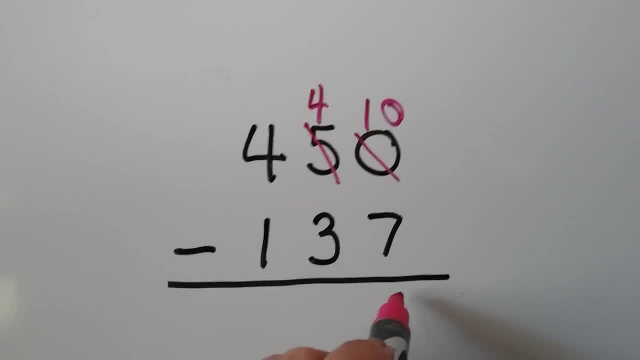 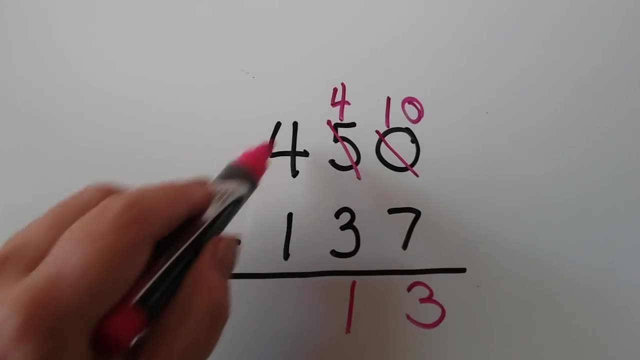 Now we have ten. take away seven, We can do that. That's a three. We have four: take away three for the tens place. That's a one. And we have four. take away one, That's a three. We have three hundred thirteen. 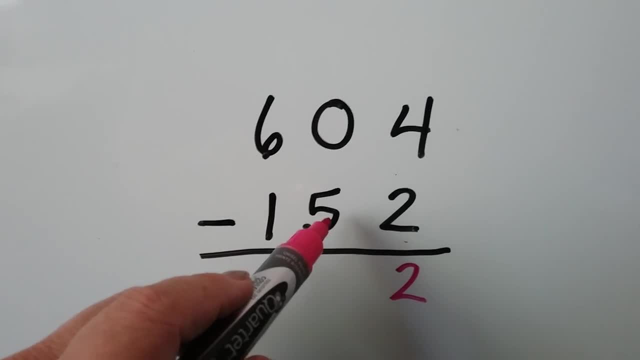 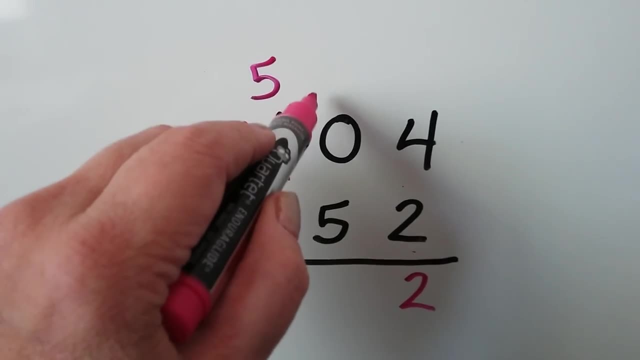 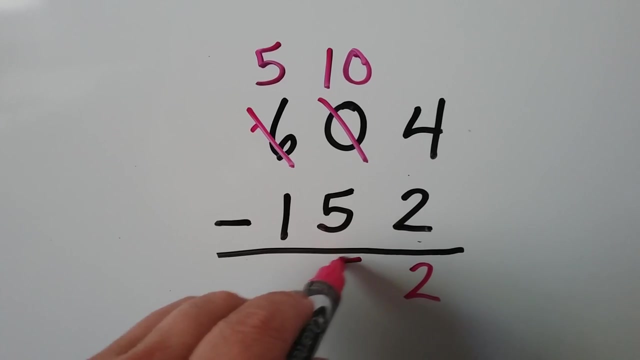 We have zero. take away five. Oh, we need to regroup because that zero is too small. This becomes a five. We give that to the tens place Ten. tens make a hundred. So we have ten tens now. Ten take away five is five, And five take away one is four. We have four hundred fifty-two. 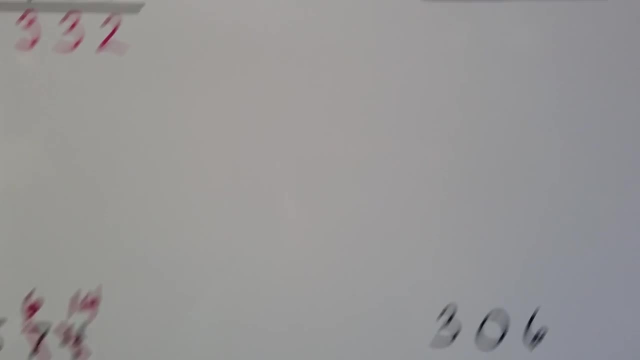 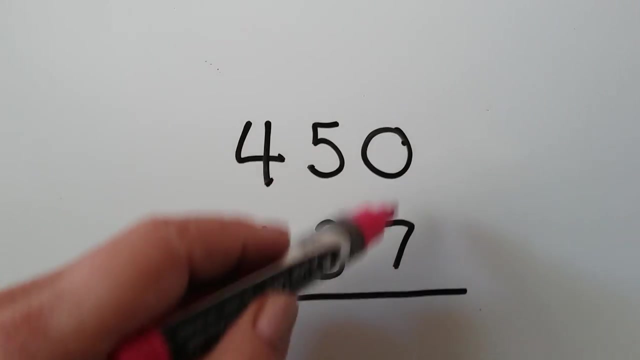 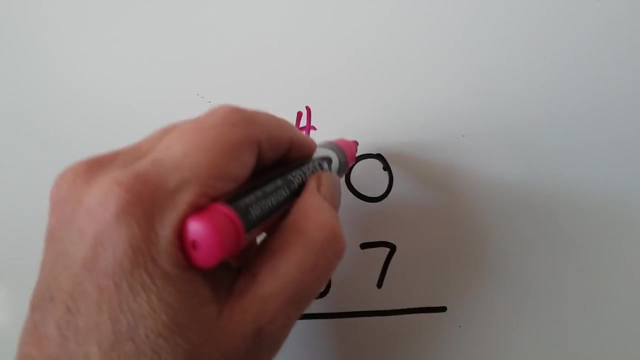 Alright, let's try it again. We're going to get lots of practice. We have four hundred fifty And we need to subtract one hundred thirty-seven. We can't have zero and take seven away, So we're going to regroup. This is going to become a four And we're going to give that ten to the ones place. 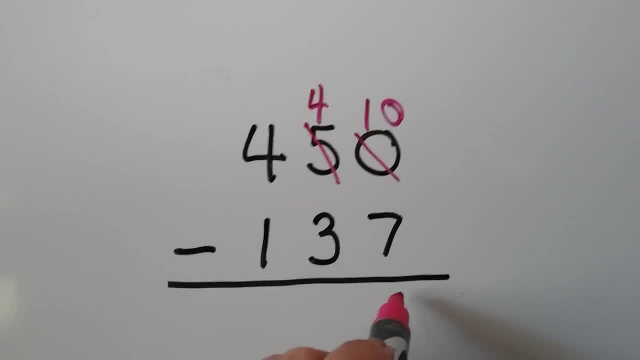 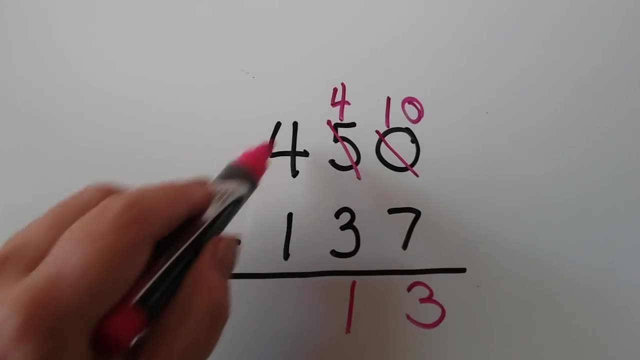 Now we have ten. take away seven, We can do that. That's a three. We have four: take away three for the tens place. That's a one. And we have four. take away one, That's a three. We have three hundred thirteen. 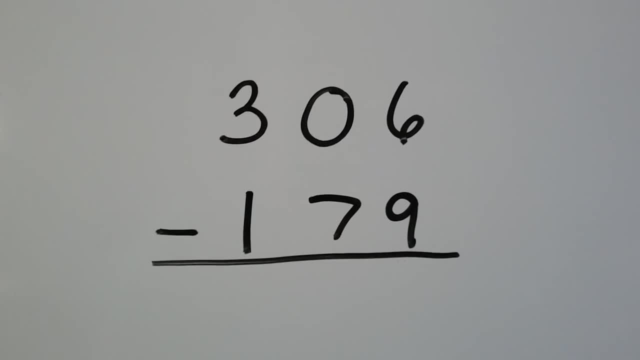 Okay, let's try it again. This one's going to be a little bit harder because we're going to have to regroup twice. We have three hundred six minus one hundred seventy-nine. We have a six and we need to take nine away. We can't do that. The nine's too big. 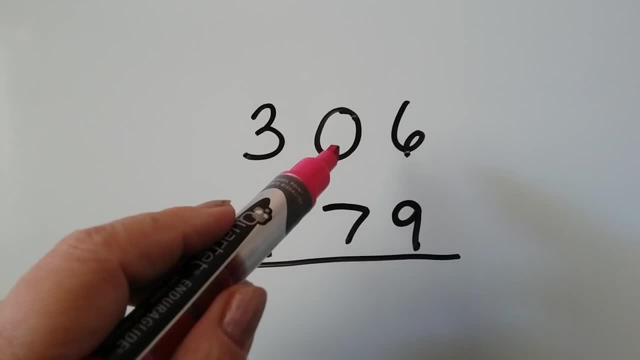 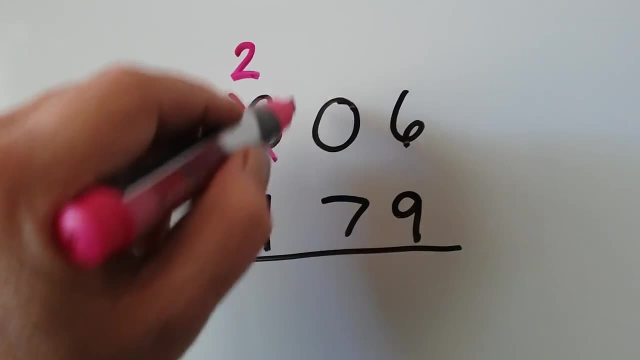 And we can't regroup from the tens place because it's a zero. So now we have to go way over to here. That becomes a two. It's one less, And instead of zero tens now we have ten tens, because ten tens make a hundred right. 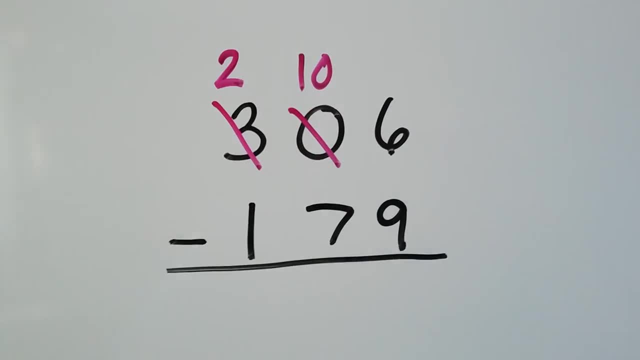 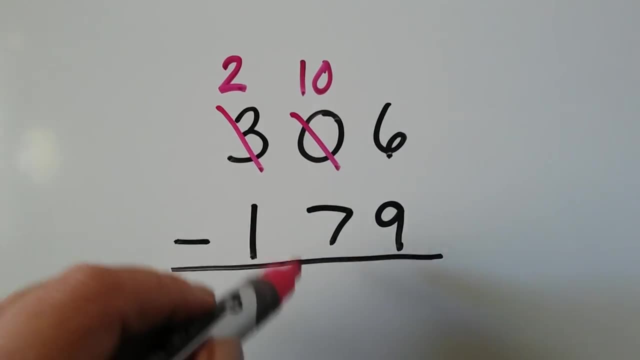 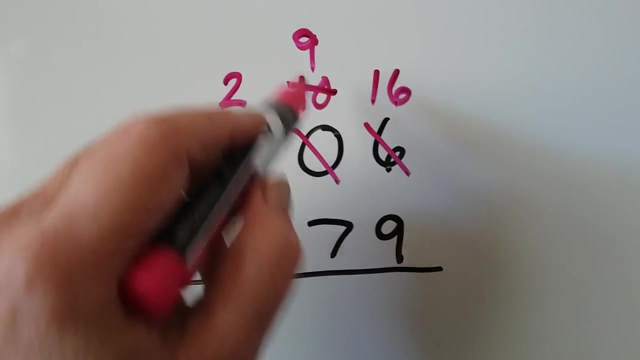 Now the ones place can be regrouped And the tens place can be regrouped because it has enough, doesn't it? So this ten is going to become a nine and this six is going to become a sixteen. We're going to give that. take one of the tens from here and give it to the ones place. 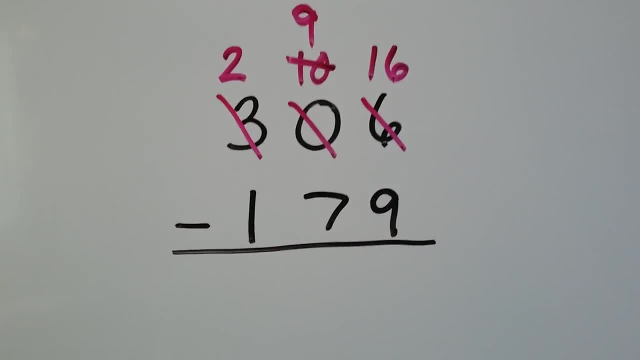 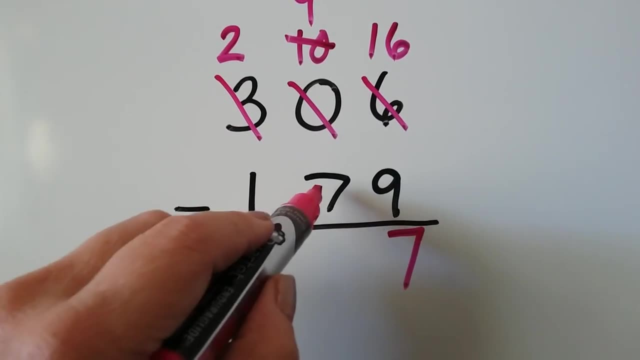 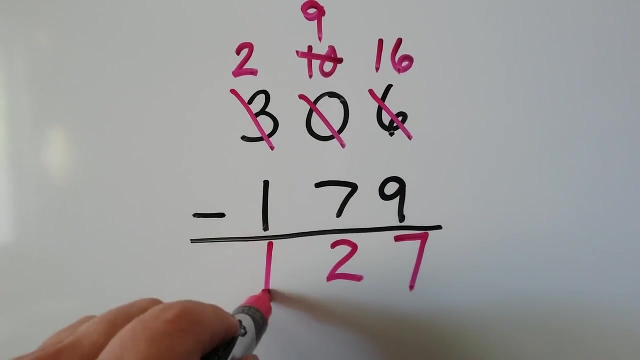 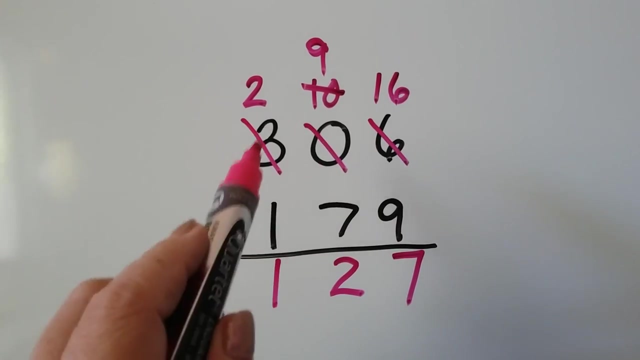 Sixteen minus nine is. do you know? That would be a seven. Nine minus seven is a two, And two minus one is one, See. So if there's a zero in the tens place and you still need to regroup, you just go to the hundreds place and regroup a couple times, See. 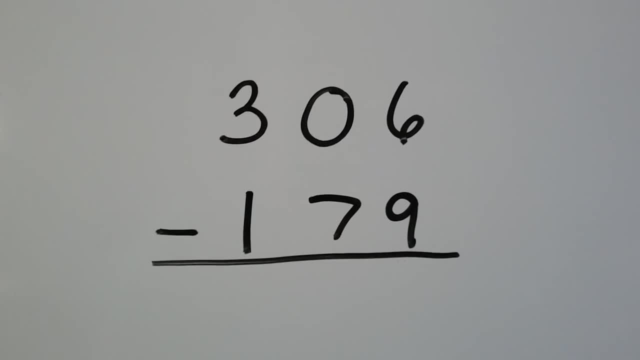 Okay, let's try it again. This one's going to be a little bit harder because we're going to have to regroup twice. We have three hundred six minus one hundred seventy-nine. We have a six and we need to take nine away. We can't do that. The nine's too big. 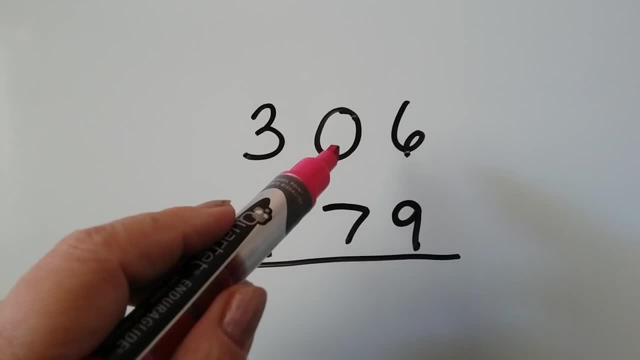 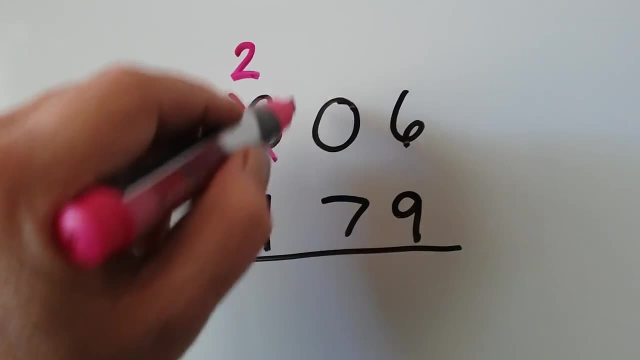 And we can't regroup from the tens place because it's a zero. So now we have to go way over to here. That becomes a two. It's one less, And instead of zero tens now we have ten tens, because ten tens make a hundred right. 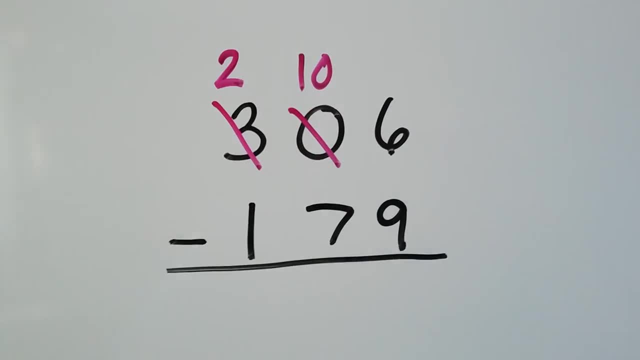 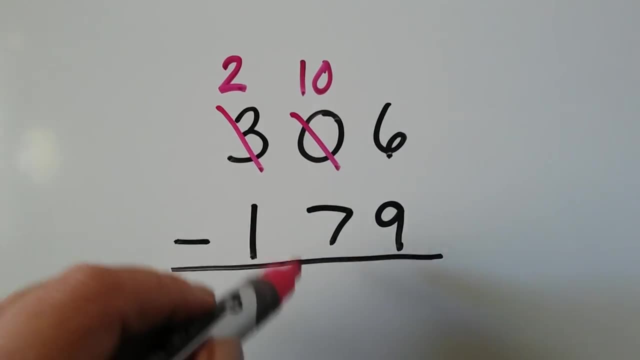 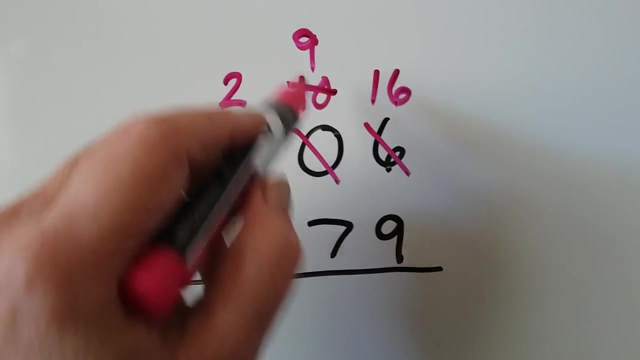 Now the ones place can be regrouped And the tens place can be regrouped because it has enough, doesn't it? So this ten is going to become a nine and this six is going to become a sixteen. We're going to give that. take one of the tens from here and give it to the ones place. 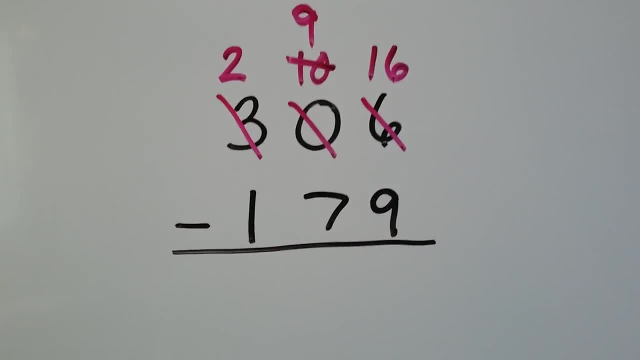 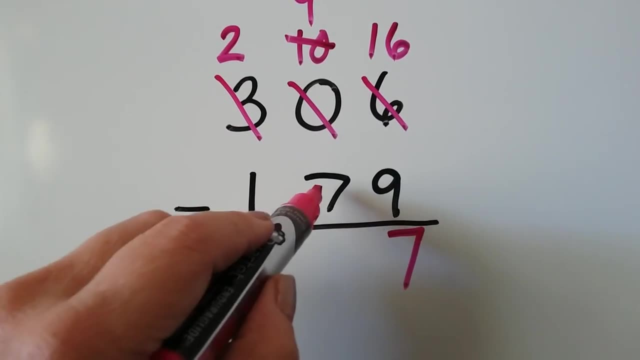 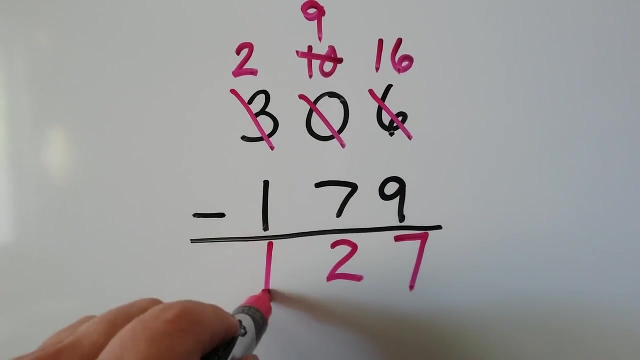 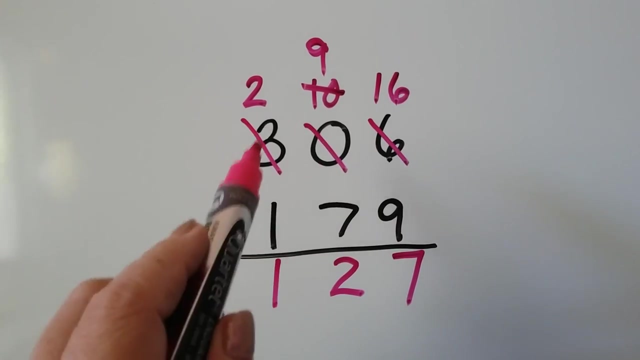 Sixteen minus nine is. do you know? That would be a seven. Nine minus seven is a two, And two minus one is one, See. So if there's a zero in the tens place and you still need to regroup, you just go to the hundreds place and regroup a couple times, See. 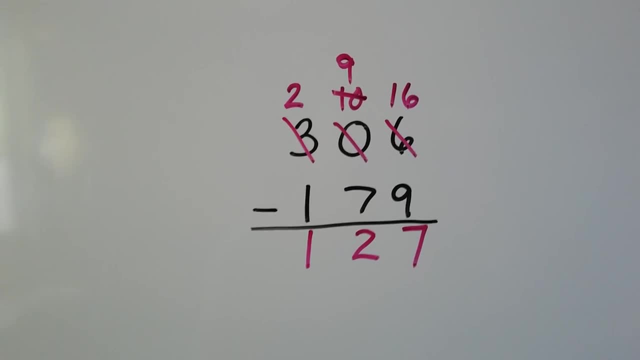 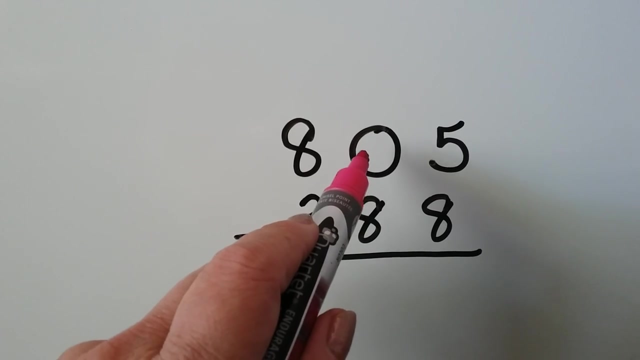 We regrouped a lot, didn't we? But that's okay, Let's try it again. We have eight hundred five minus three hundred eighty-eight. We have a five and we can't take away eight, And there's zero tens, so we can't regroup from the tens place. 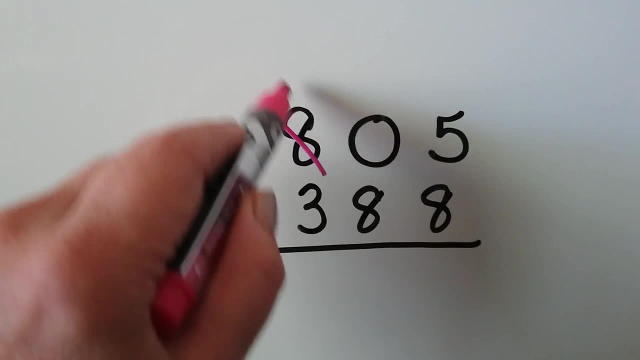 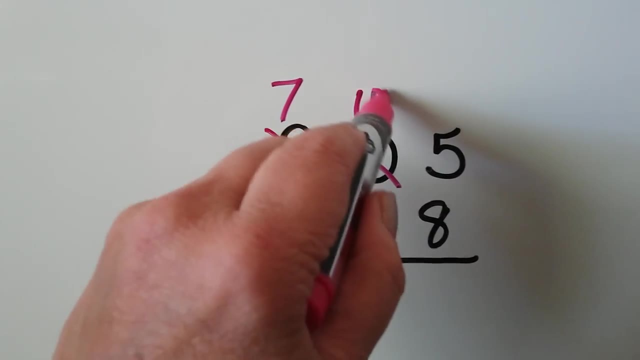 We're going to have to keep going and go to the hundreds place. That's going to become a seven. So now instead of zero tens, we have ten tens, because ten tens make one hundred. That's what we regrouped from the hundreds place. 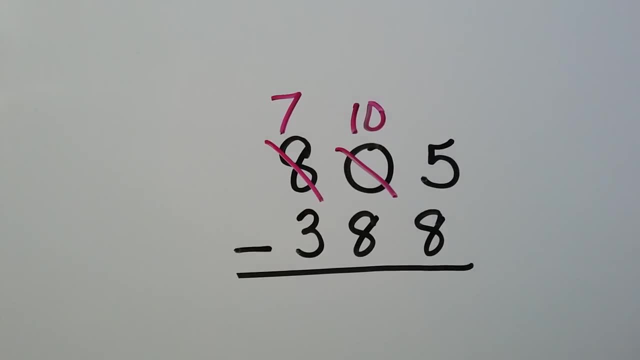 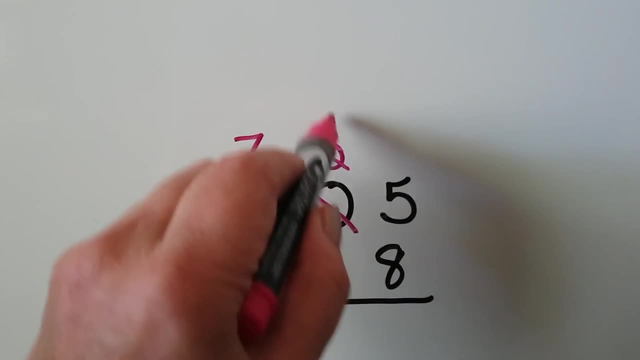 We took one of the hundreds away and gave it to the tens as ten tens. right Now we can regroup and give some to the ones place. So the ten is going to become a nine And we're going to give it to the ones place. 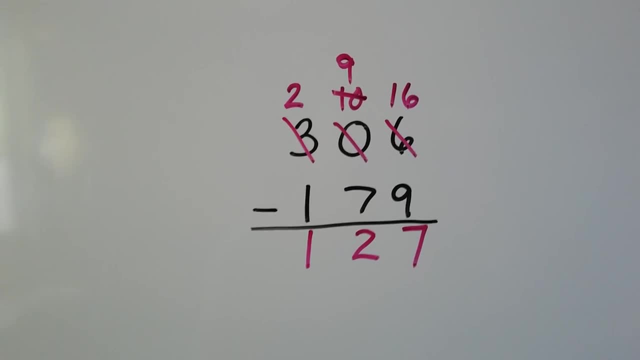 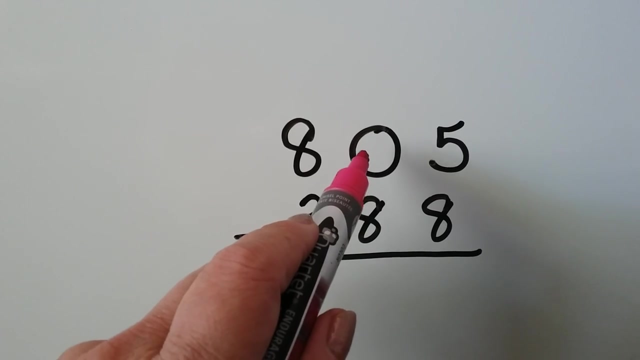 We regrouped a lot, didn't we? But that's okay, Let's try it again. We have eight hundred five minus three hundred eighty-eight. We have a five and we can't take away eight, And there's zero tens, so we can't regroup from the tens place. 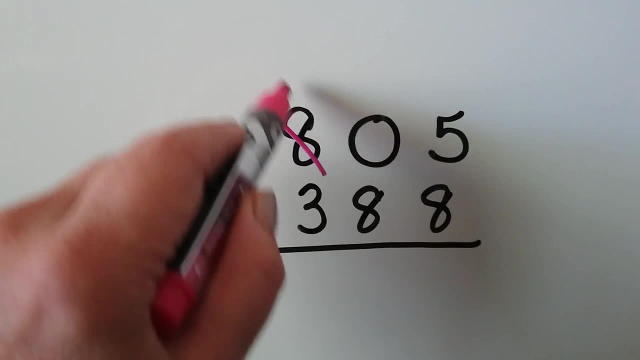 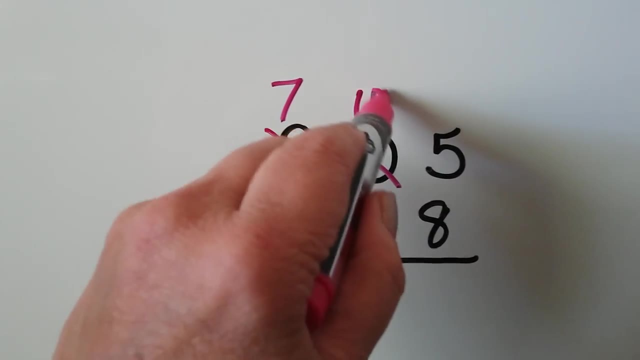 We're going to have to keep going and go to the hundreds place. That's going to become a seven. So now instead of zero tens, we have ten tens, because ten tens make one hundred. That's what we regrouped from the hundreds place. 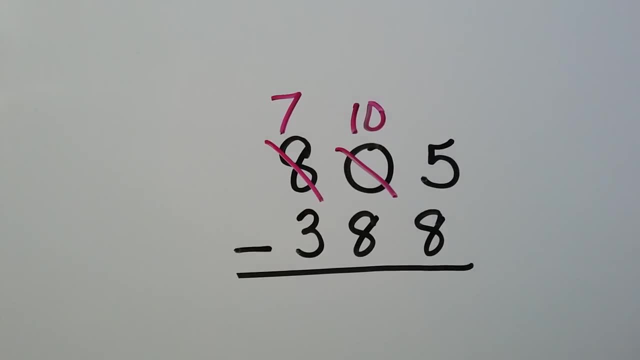 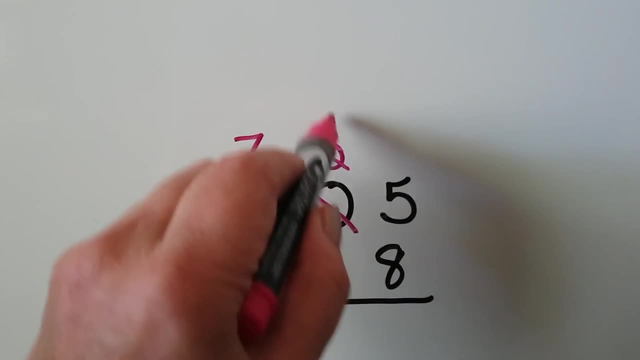 We took one of the hundreds away and gave it to the tens as ten tens. right Now we can regroup and give some to the ones place. So the ten is going to become a nine And we're going to give it to the ones place. 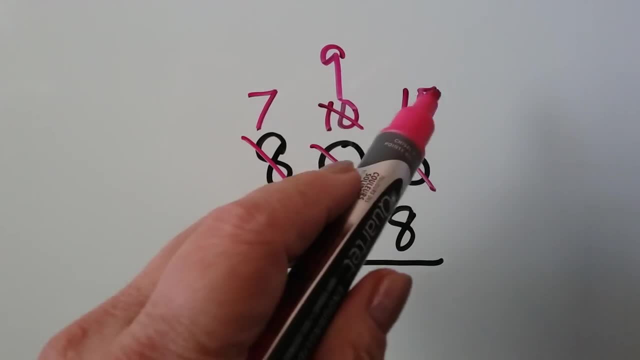 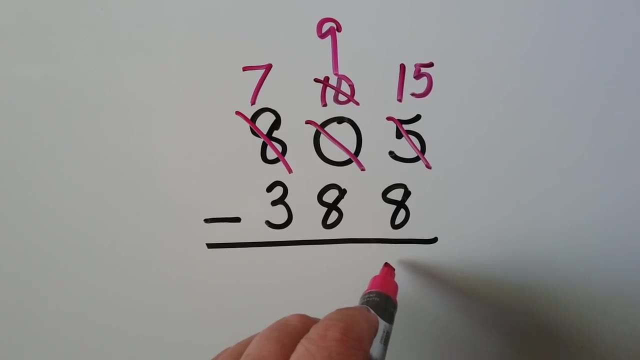 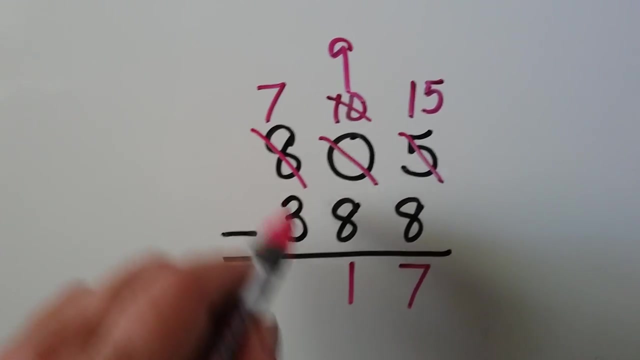 So instead of five ones, we have fifteen ones. Fifteen take away eight is, Do you know? It would be a seven. Nine take away eight. That's an easy one, isn't it? That's a one, And seven take away three is. 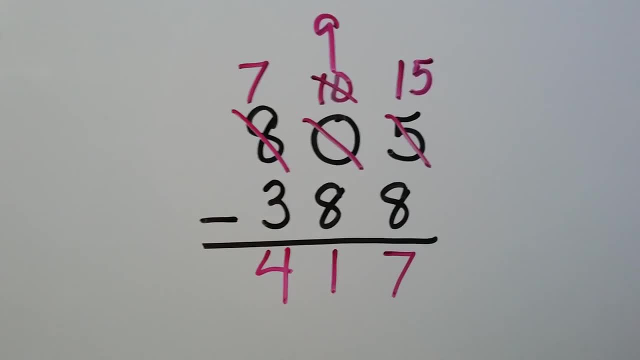 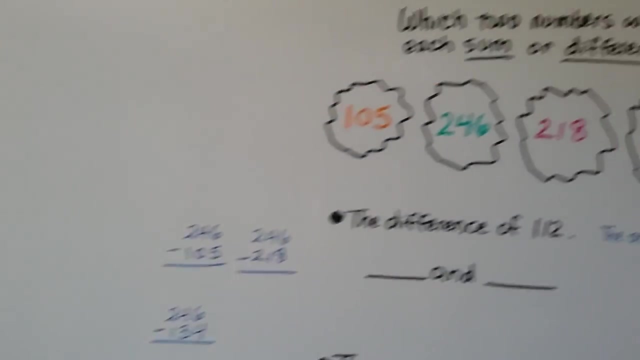 A four, We have four hundred seventeen, So we had to regroup a couple times. It's no different than regrouping once You're just doing it again. It's not harder, It just takes a little longer. Let's try some problem solving. 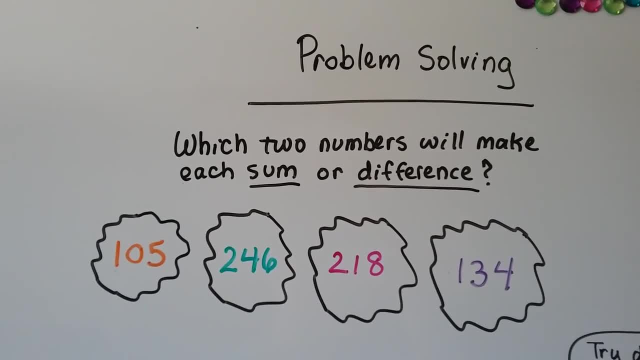 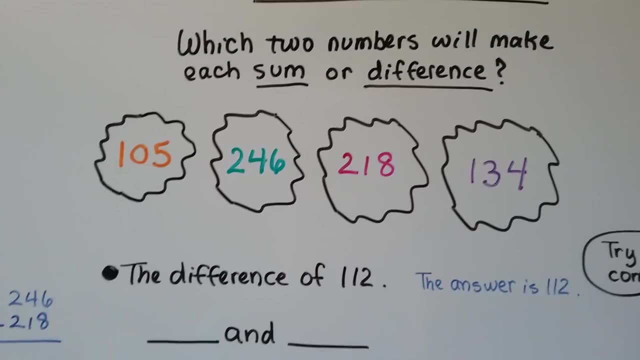 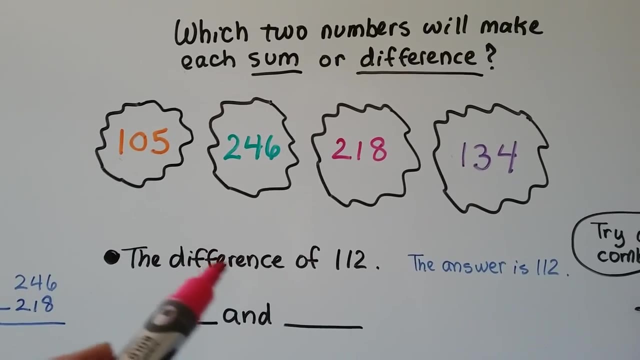 It says which two numbers will make each sum or difference. We have one hundred five, two hundred forty-six, two hundred eighteen and one hundred thirty-four. We need to find the difference of one hundred twelve. That means because difference is the answer in subtraction. 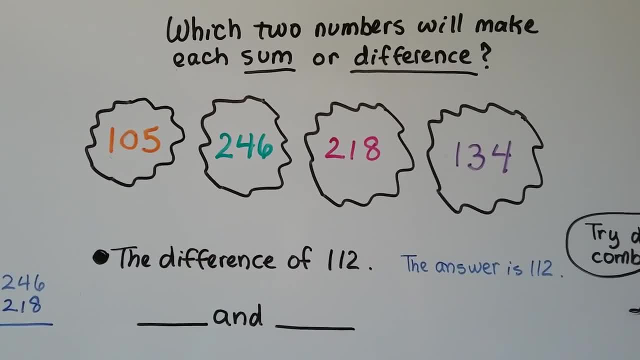 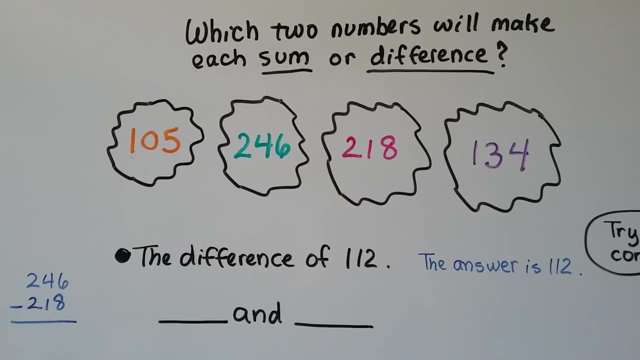 that means that the answer is one hundred twelve And because it's a difference, we know it's going to be a subtraction problem. So we need to find which two of these numbers are going to equal one hundred twelve when you subtract one from the other. 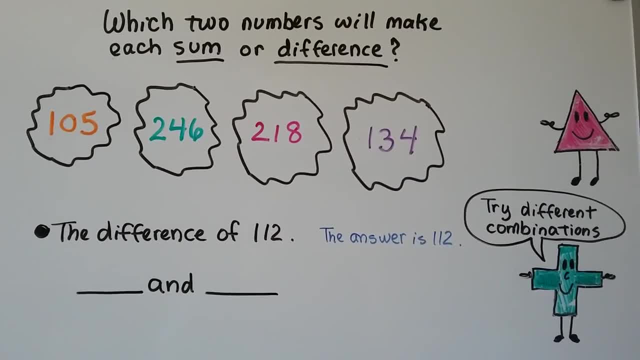 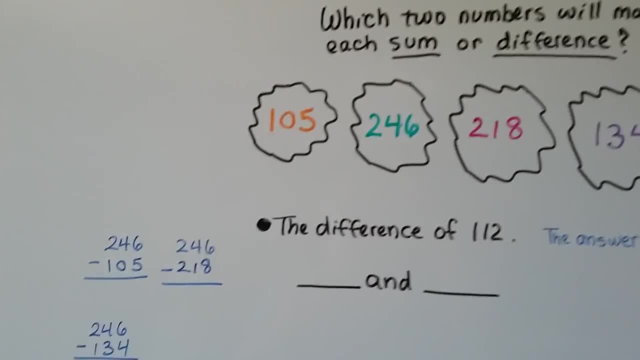 And the only way to do it is to try different combinations. See, the little plus sign is telling us: just try different combinations. So we can try two hundred forty-six minus one hundred five. We could try that: Two hundred forty-six minus one hundred five. 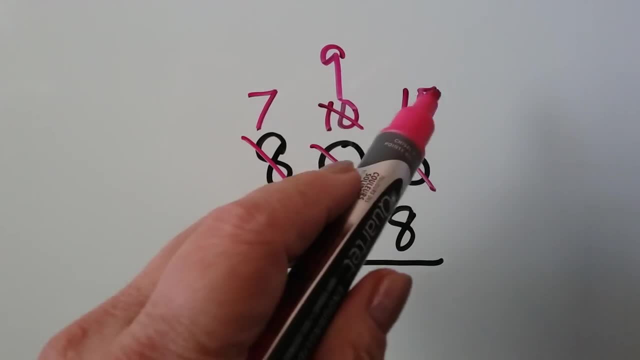 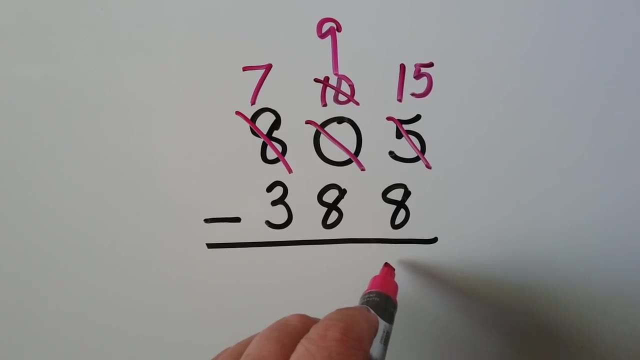 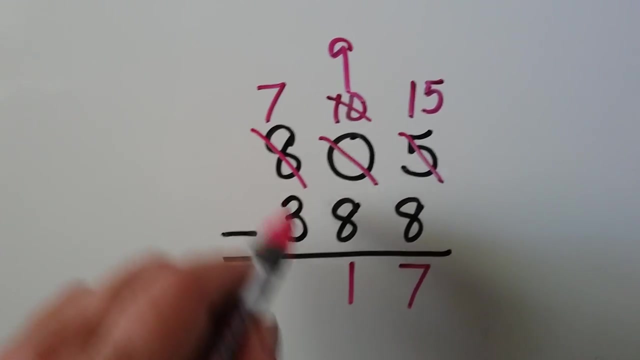 So instead of five ones, we have fifteen ones. Fifteen take away eight is, Do you know? It would be a seven Nine take away eight. That's an easy one, isn't it? That's a one. And seven take away three is a. 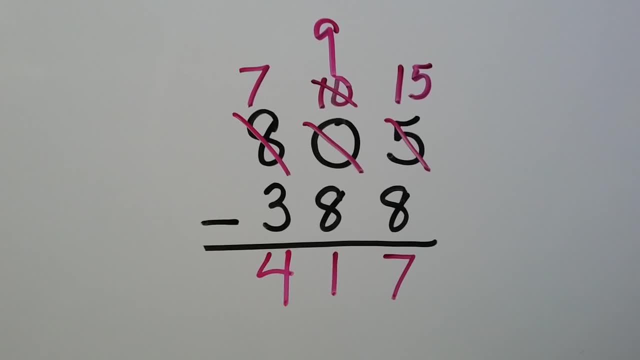 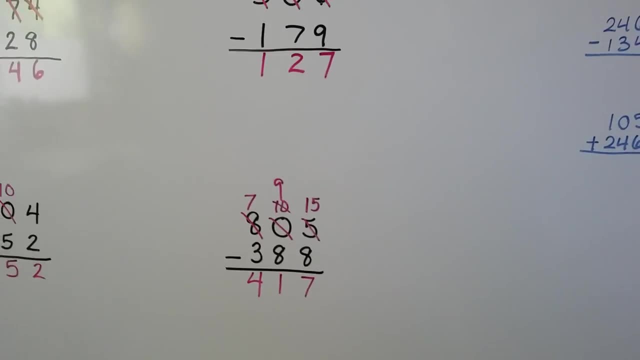 A four, We have four hundred seventeen, Okay, So we had to regroup a couple times. Alright, It's no different than regrouping once. You're just doing it again. Okay, It's not harder, It just takes a little longer. 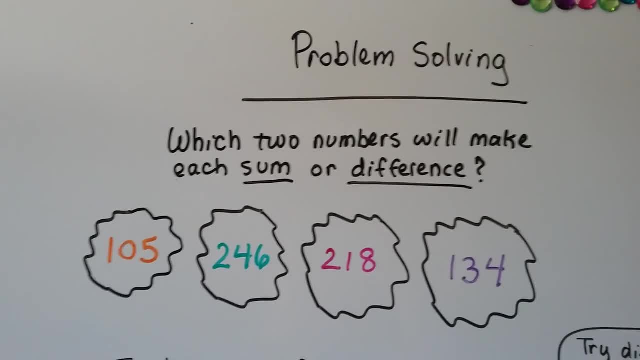 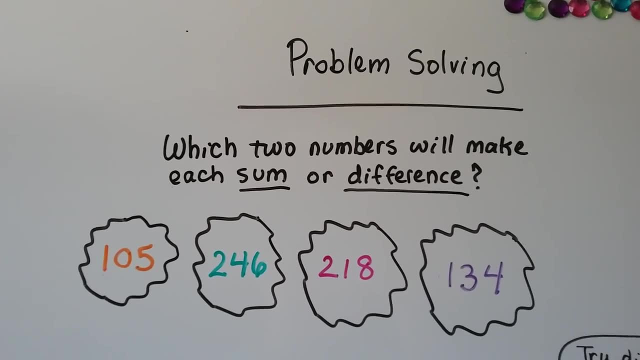 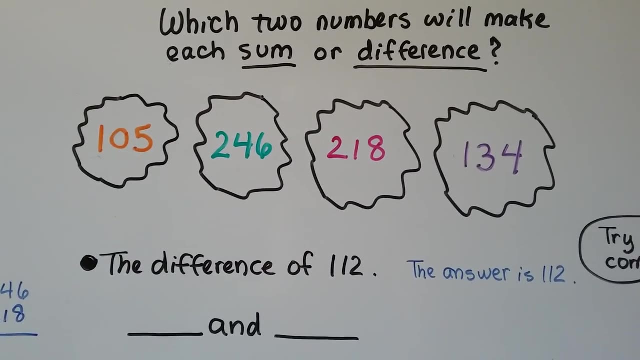 Okay, Let's try some problem solving. It says which two numbers will make each sum or difference. We have one hundred five, two hundred forty-six, two hundred eighteen and one hundred thirty-four. We need to find the difference of one hundred twelve. 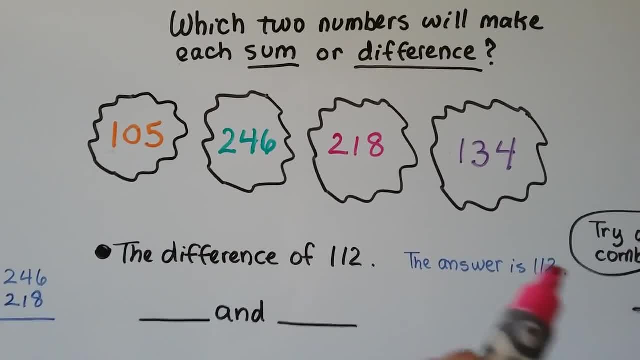 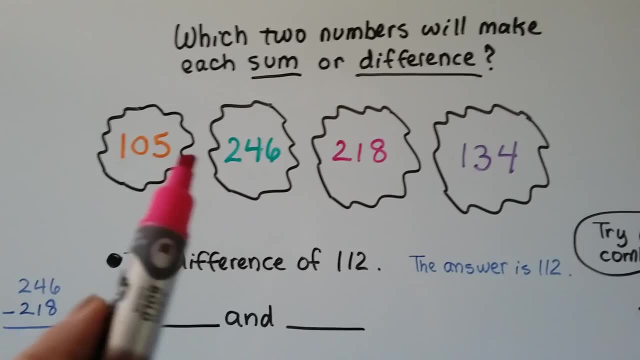 That means because difference is the answer, in subtraction, that means that the answer is one hundred twelve. And because it's a difference, we know it's going to be a subtraction problem. So we need to find which two of these numbers are going to equal one hundred twelve when you subtract one from the other. 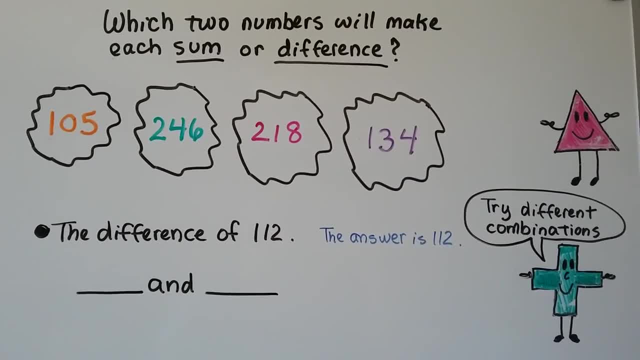 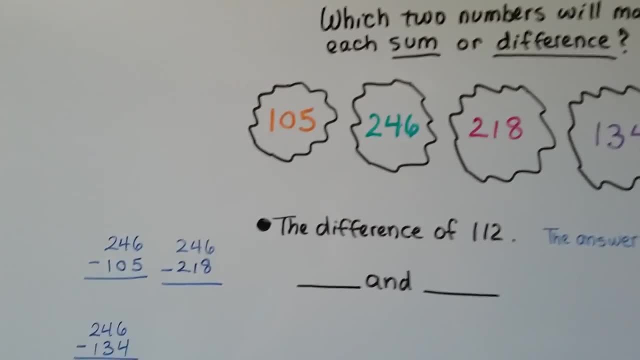 And the only way to do it is to try different combinations. See little plus signs telling us Different combinations. So we can try two hundred forty-six minus one hundred five. We could try that Two hundred forty-six minus one hundred five, Six minus five is a one. 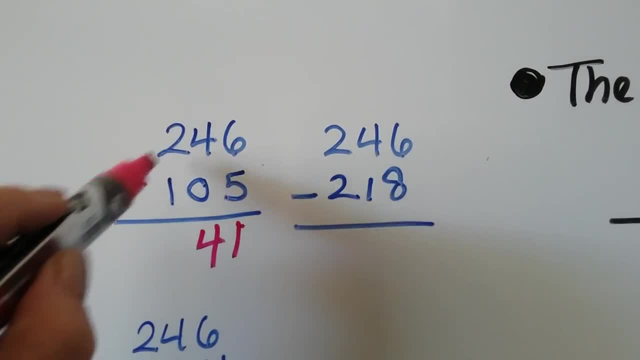 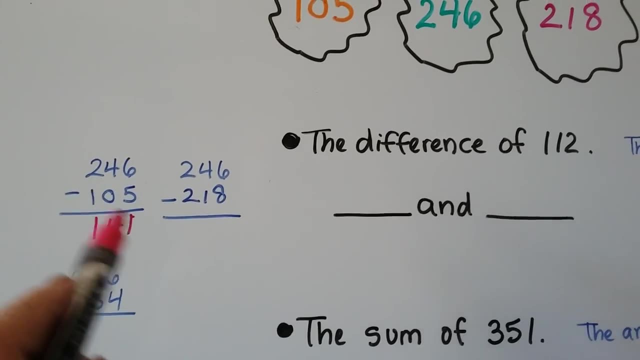 Four minus zero is four. Two minus one is one. Well, that's a hundred and forty-one, That's not a hundred and twelve, So that's not the right combination. Let's try two hundred forty-six minus two hundred eighteen. Let's try this: one minus this one. 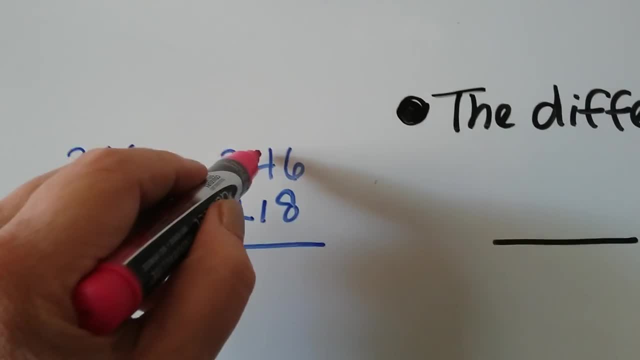 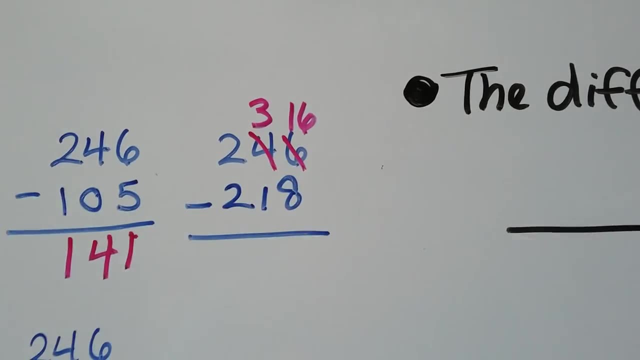 We have six And we need to take away eight and we can't. So we regroup. That becomes a three, That becomes a sixteen, Right, Because we gave a ten to the ones place. Sixteen minus eight. Well, eight plus eight is sixteen. 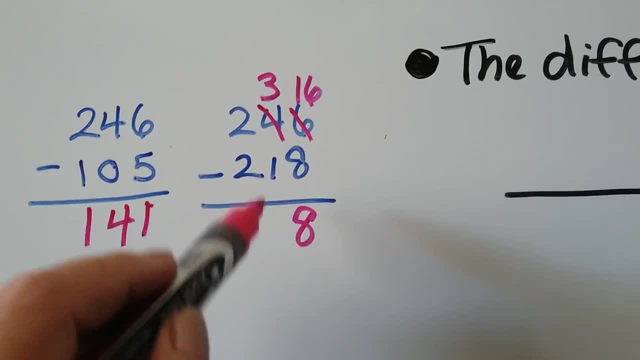 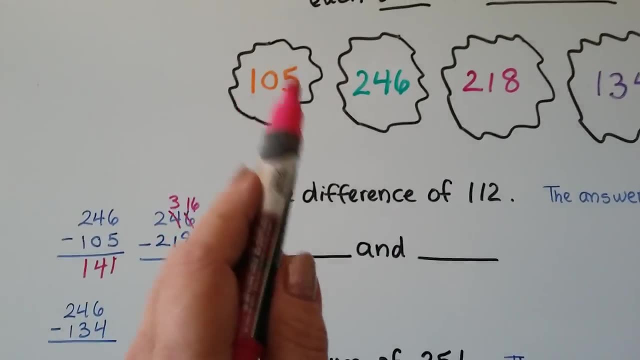 That's a double, So we know that's an eight. Three minus one is a two, And two minus two is a zero. Hmm, That's only twenty-eight. So two hundred forty-six minus one hundred five didn't work. Two hundred forty-six minus two hundred eighteen didn't work. 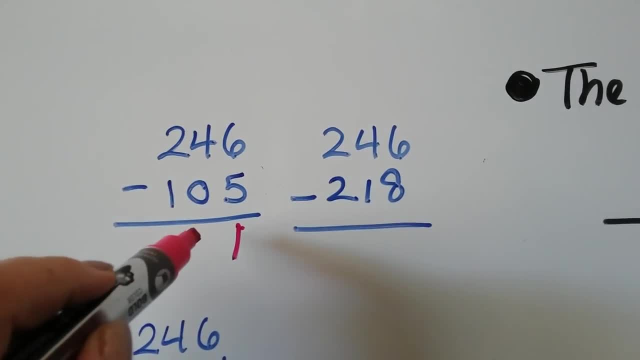 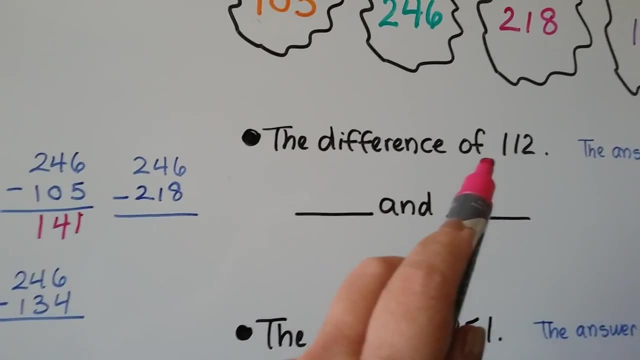 Six minus five is a one. Four minus zero is four. Two minus one is one. Well, that's a hundred and forty-one. That's not a hundred and twelve. So that's not the right combination. Let's try: two hundred forty-six minus two hundred eighteen. 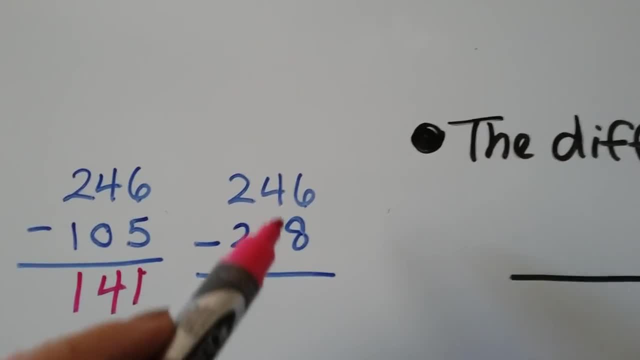 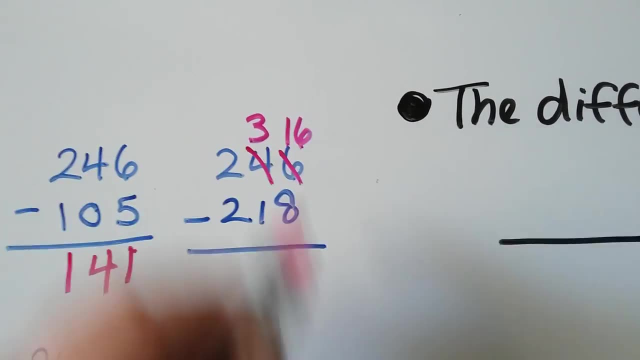 Let's try this one minus this one. We have six and we need to take away eight And we can't. So we regroup, That becomes a three, That becomes a sixteen Right, Because we gave a ten to the ones place. 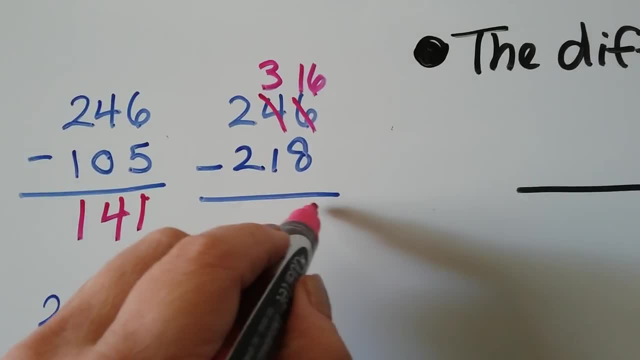 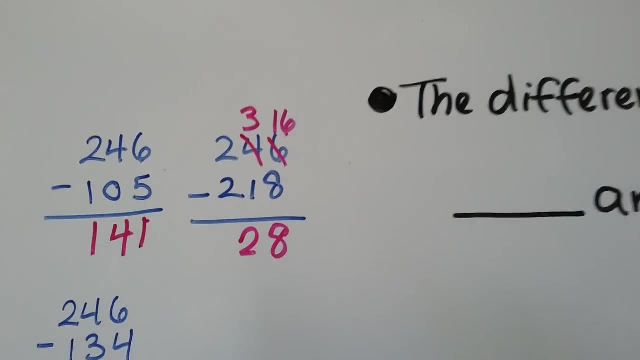 Sixteen minus eight. Well, eight plus eight is sixteen, That's a double, So we know that's an eight. Three minus one is a two, And two minus two is a zero. Hmm, That's only twenty-eight. So two hundred forty-six minus one hundred five didn't work. 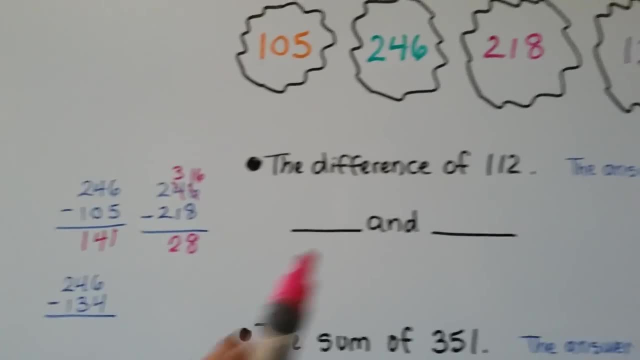 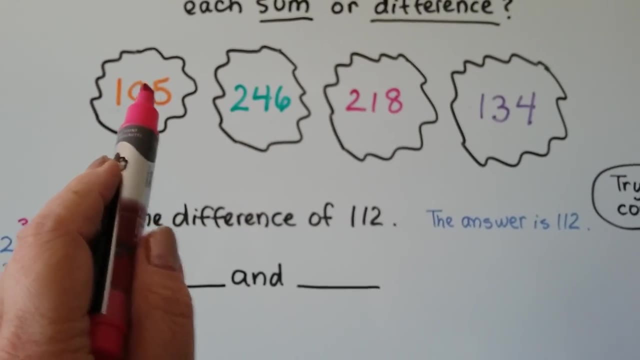 Two hundred forty-six minus two hundred eighteen didn't work. Let's try two hundred forty-six Minus the one hundred thirty-four. It could also be two hundred eighteen minus one hundred five, Couldn't it? Or two hundred eighteen minus one hundred thirty-. 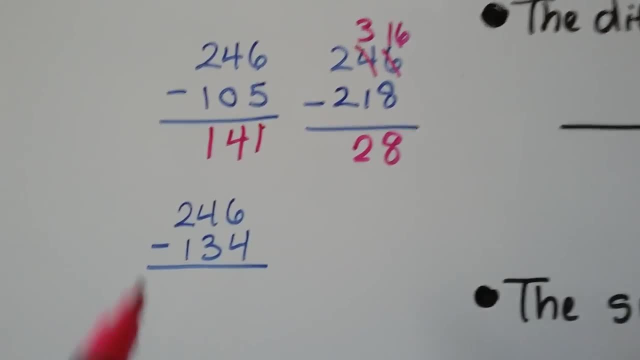 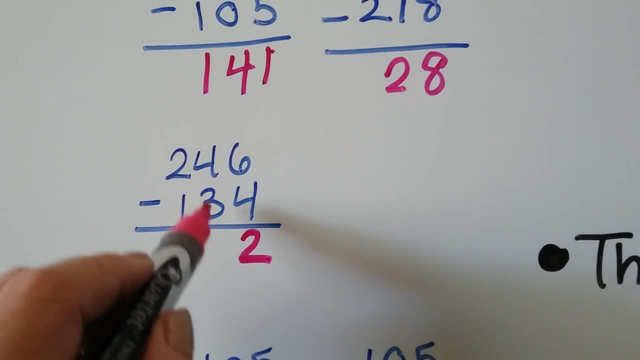 We could even try half- We might even have to do that, Right? So let's try. two hundred forty-six minus one hundred thirty-four. Six minus four is a two. Four minus three is a one. Oh, look at this. Two minus one is a one. 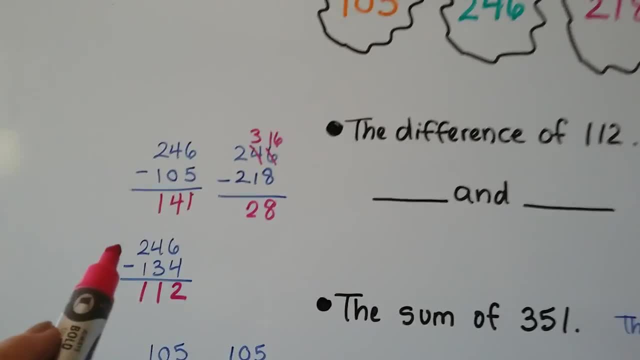 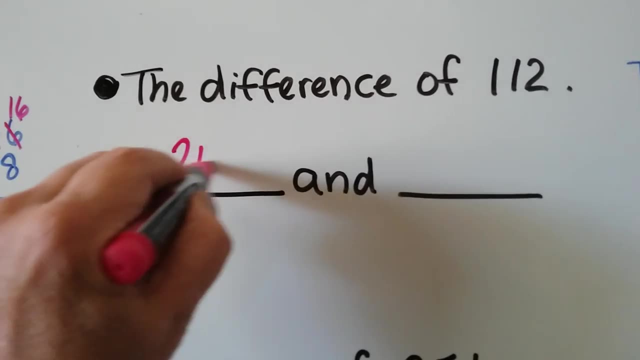 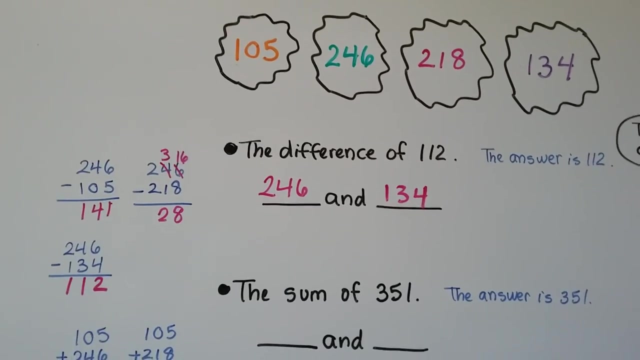 It is one hundred twelve. So we know the two numbers are two hundred forty-six and one hundred thirty-four. Two hundred forty-six and one hundred thirty-four. So the only way we could figure out which would make the difference of one hundred twelve was by doing math on the side. 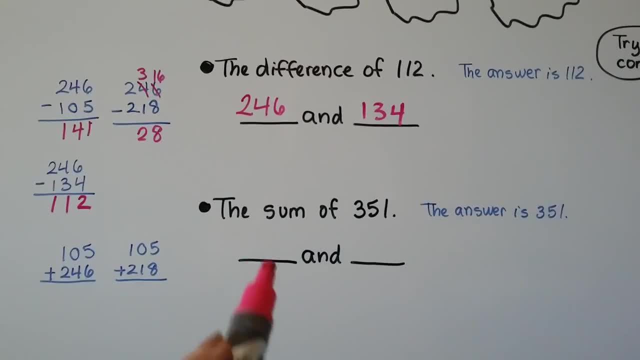 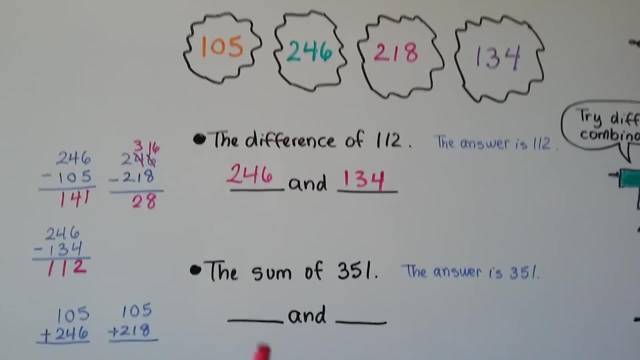 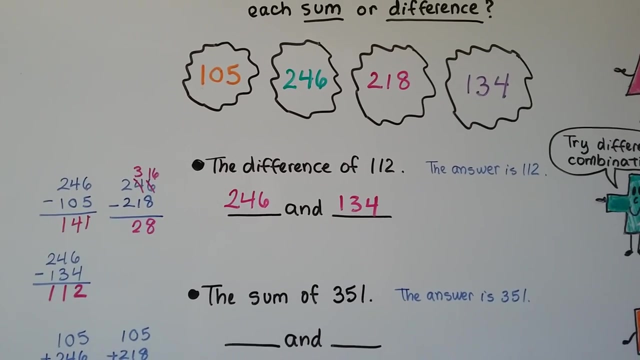 and just trying different combinations. Okay now, this one says the sum of three hundred fifty-one. So two of these numbers, when added together- because a sum is an answer in addition, isn't it? Two of these numbers added together are going to give us a sum of three hundred fifty-one. 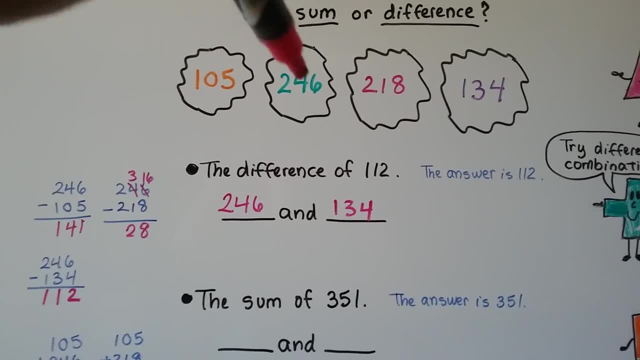 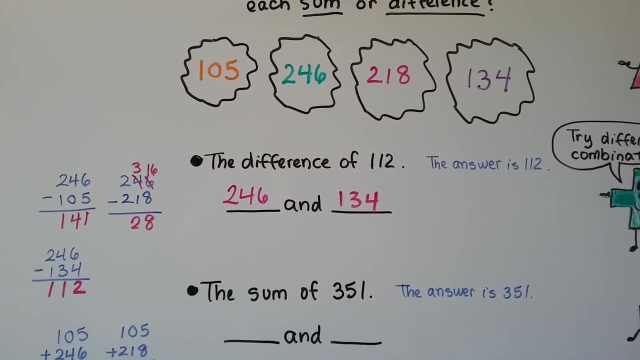 We have to figure out which ones they are. If we add these two together, will that give us three hundred fifty-one. If we add these two together, will that do it Or will this do it? So we need to try different combinations. 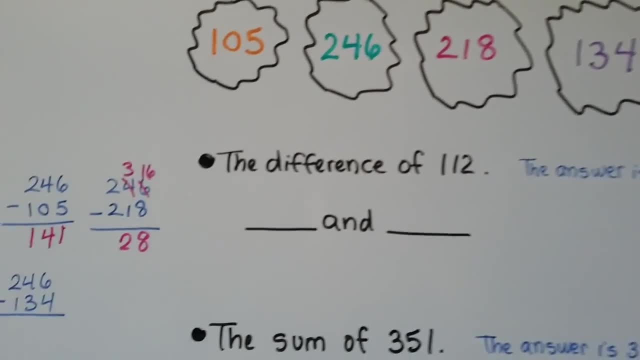 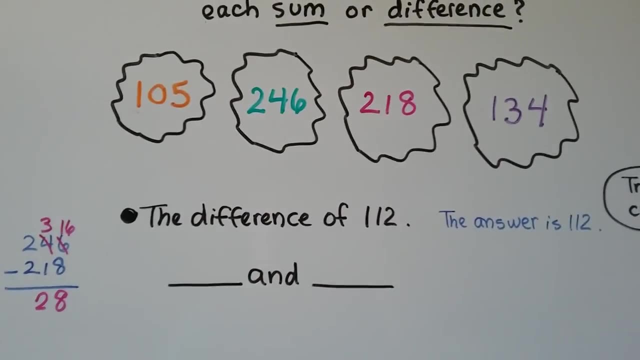 Let's try two hundred forty-six minus the one hundred thirty-four. It could also be two hundred eighteen minus one hundred five, couldn't it? Or two hundred eighteen minus one hundred thirty- We could even try half- We might even have to do that right. 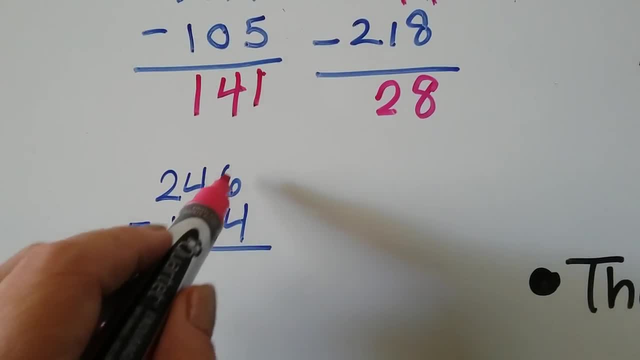 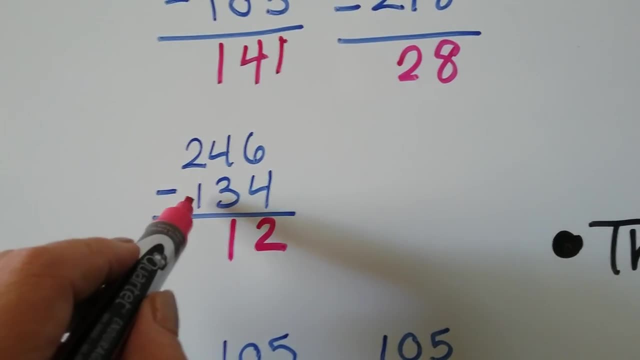 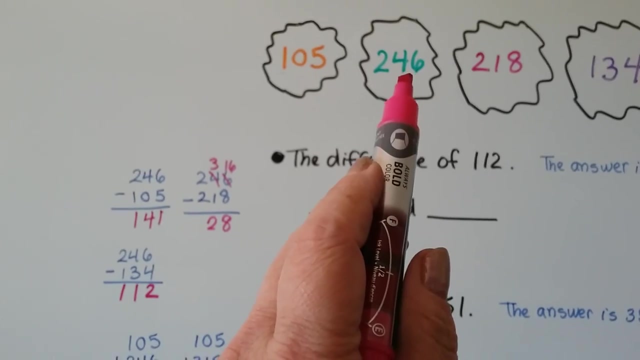 So let's try. two hundred forty-six minus one hundred thirty-four. Six minus four is a two. Four minus three is a one. Oh, look at this. Two minus one is a one, It is one hundred twelve. So we know. the two numbers are two hundred forty-six and one hundred thirty-four. 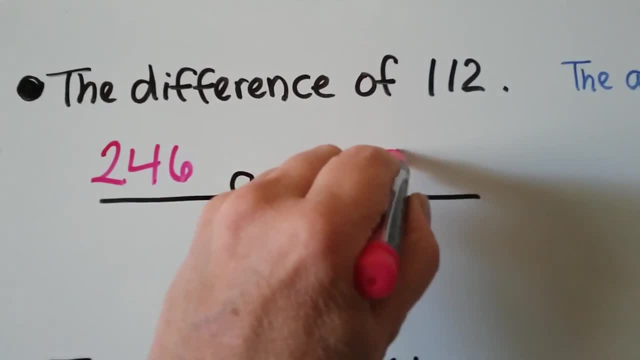 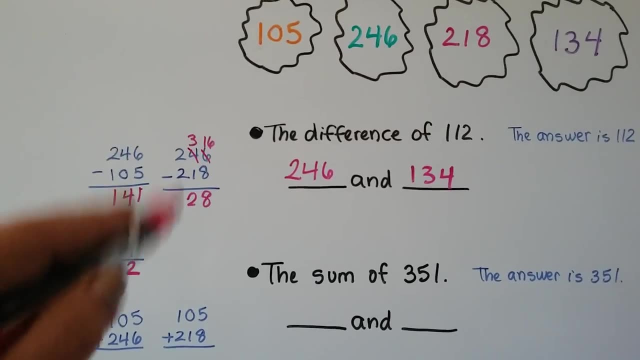 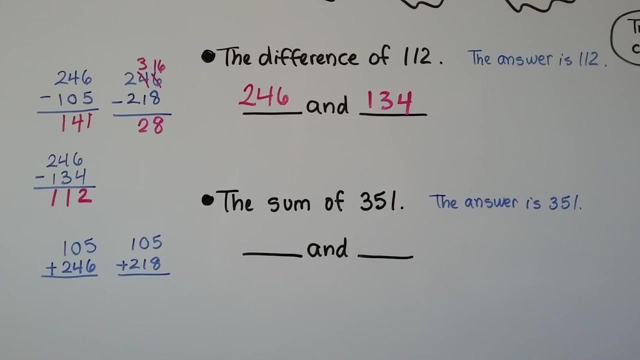 Two hundred forty-six and one hundred thirty-four. So the only way we could figure out which would make the difference of one hundred twelve was by doing math on the side and just trying different combinations. Okay, now this one says the sum of three hundred fifty-one. 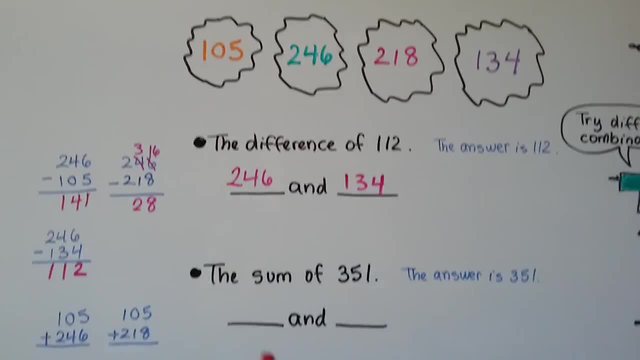 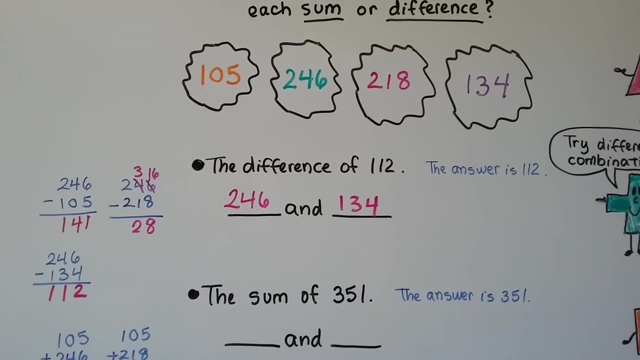 So two of these numbers when added together- because a sum is an answer in addition, isn't it? Two of these numbers added together are going to give us a sum of three hundred fifty-one. We have to figure out which ones they are. 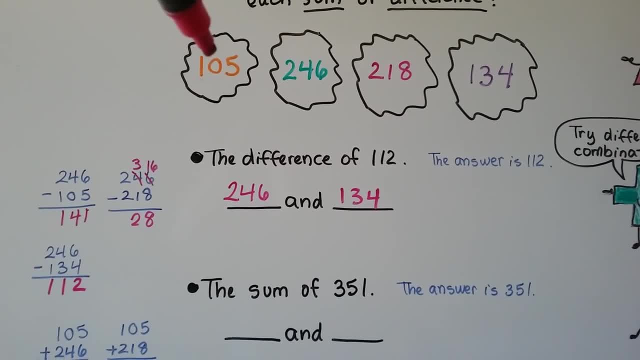 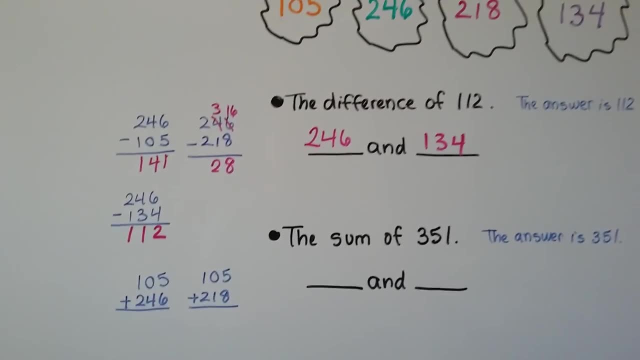 If we add these two together, will that give us three hundred fifty-one? If we add these two together, will that do it Or will this do it? So we need to try different combinations. Let's try one hundred five and two hundred forty-six, the first two numbers. okay. 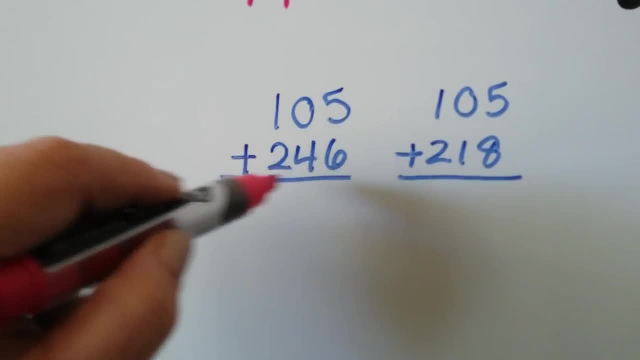 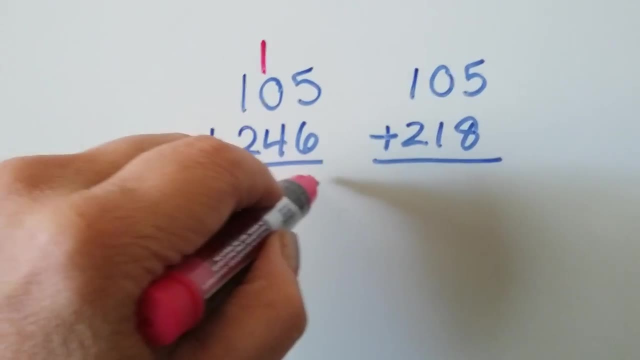 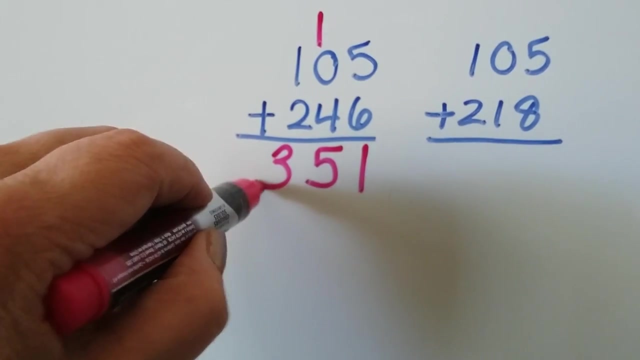 So we have five hundred fifty-six. We have five because we're adding now five plus six. Well, five plus five is ten, so five plus six is eleven. We regroup the one and put the one down. One plus zero plus four is five, and one plus two is three. 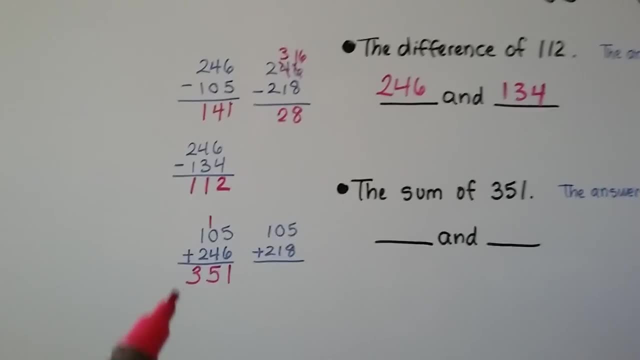 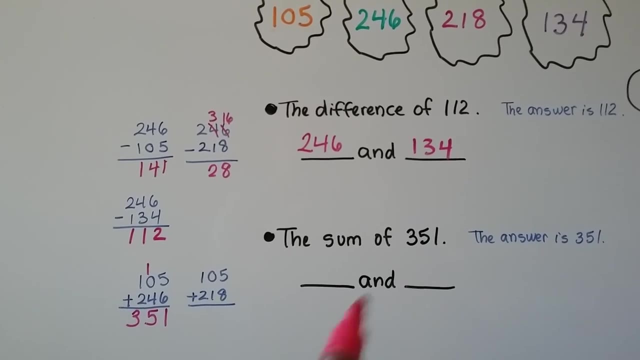 Look at that. we got lucky. The very first two numbers we tried ended up being the right ones. It is three hundred fifty-one, So we know the answer is the two numbers that will give us a sum of three hundred fifty-one. 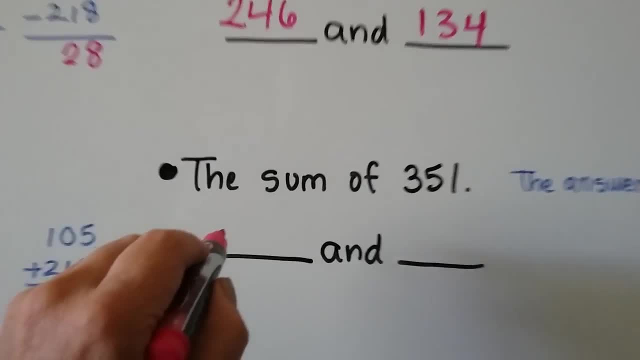 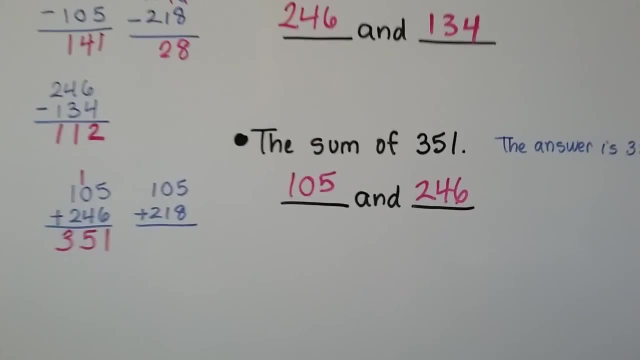 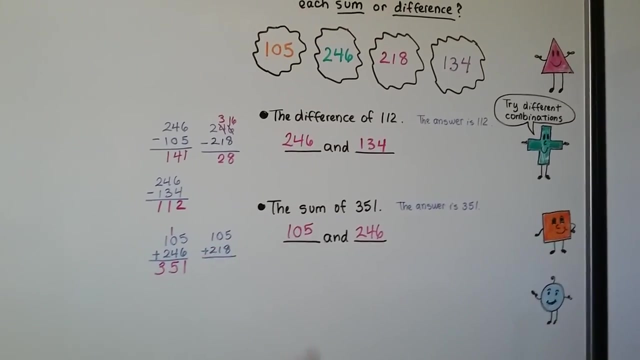 is one hundred five and two forty-six, One hundred five and two hundred forty-six, And the only way to find the answer to this problem was to do guess and check right. We had to keep trying different combinations until we got the right answers, alright.